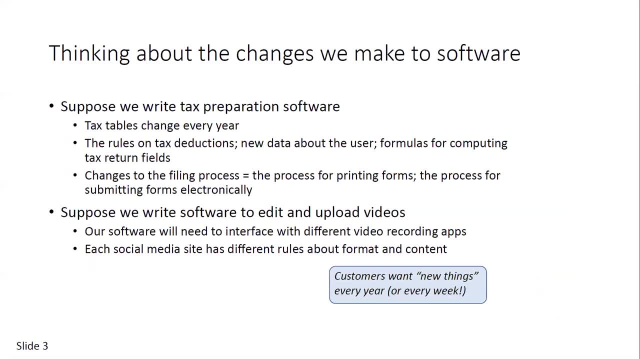 and forth. All right. So thinking about the changes we make to software? right, Suppose that we're in the business of creating tax preparation software. What changes? Well, tax tables change every year. The rules on tax deductions change. Maybe we have new. 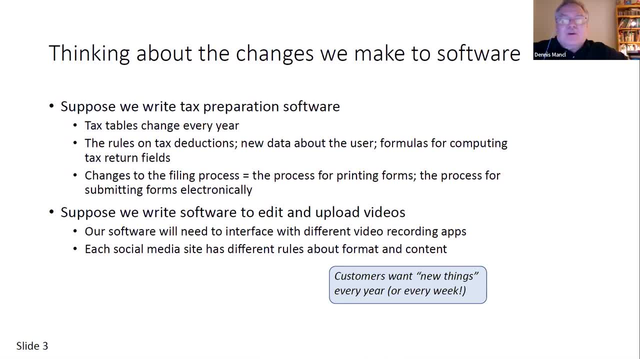 information about the user that we're maintaining. We have changes in the formulas for computing tax return fields And we might have changes to the filing process right. Changes in the printed forms. changes to the electronic submission process: Okay, Ah, so oops, sorry. Another area, right. We may be building applications to. 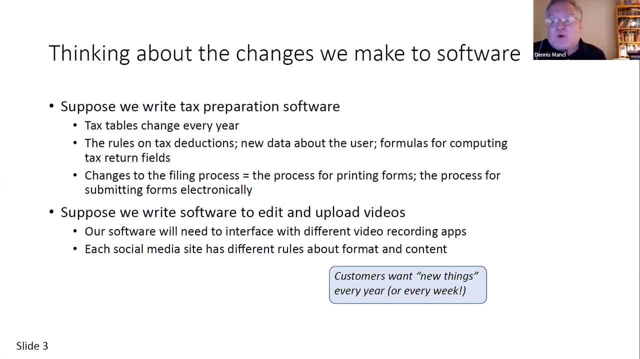 help people create and post online videos. right, And it will lead to work with various kinds of recording video recording apps. right, And those, of course, are changing all the time. right, It seems like you have a new video recording application each month, right, And for uploading. 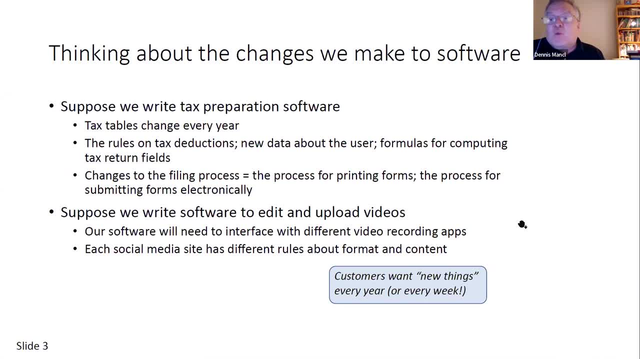 right, each social media site has different rules about the way that their stuff works. Okay, Hold on here. I am going to just take a look here, Let's see. All right, So I'm going to try to do this in a slightly different way, Because somebody is. 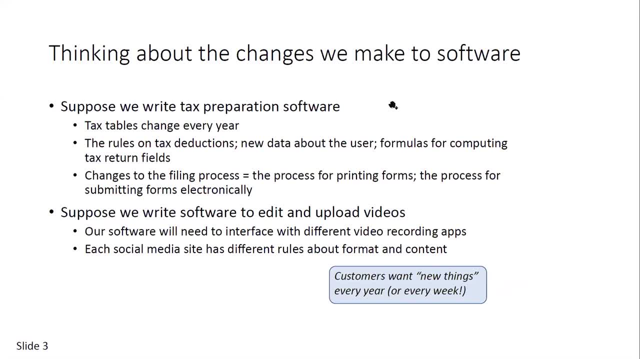 Here we go. Maybe that's it Okay. Good, All righty, Okay. So it's inevitable in these kinds of applications that we're using these things. This is just a a very simple application- tax preparation, video editing- that we're going to have changes right. Here's another one which 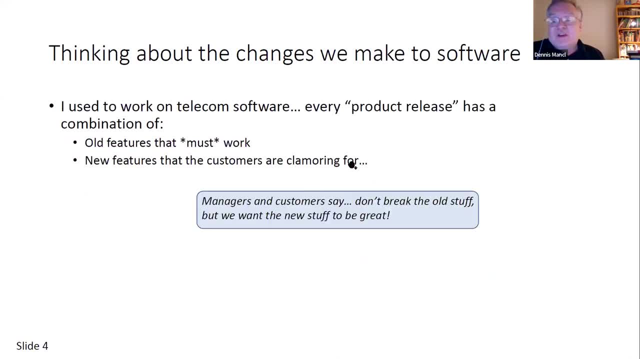 is close to my heart, which is telecom software. I used to work in this industry, right, I used to work on the development of software for various kinds of telecom operations. You know we would do, you know network management systems and so on, And customer managers and customers always. 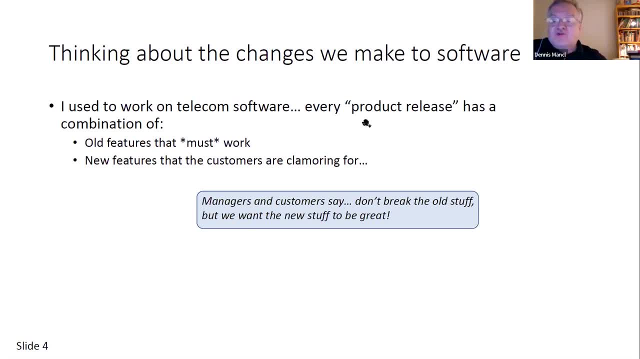 wanted something new, But of course the old features must still work. We had things like provisioning alarms, event logs that we're processing and network management tools looking for potential bottlenecks. Well, management wanted the new stuff to be great, But sometimes we had to. 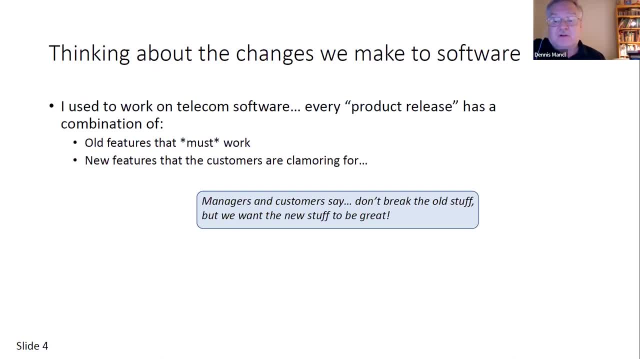 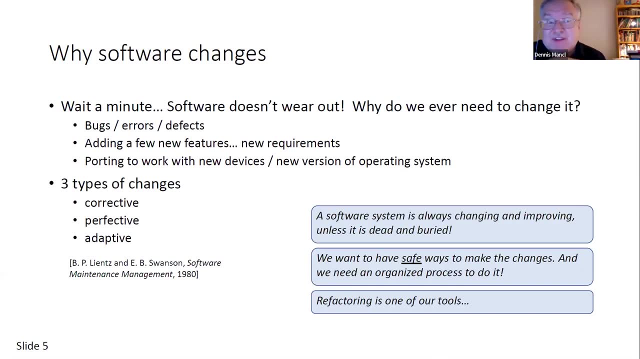 do some work to shore up the old stuff, right? So wait a minute, I thought software doesn't wear out. It's the advantage of software over hardware, right? You know you don't actually have bit decay, right? Why do we ever need to change software? Well, it's because some of the 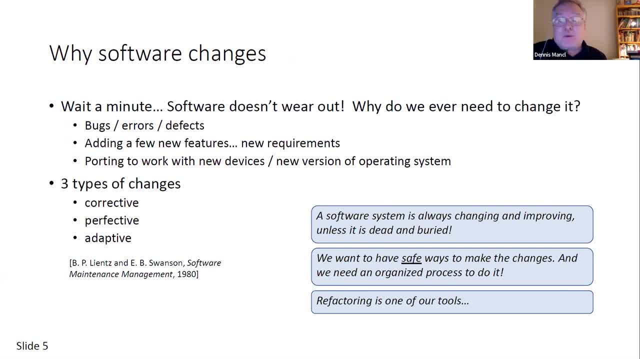 changes are related to bug fixes. You know there's problems that we had when we actually originally developed the application And sometimes it's new requirements that come in that we didn't know about last year when we were building the software right. 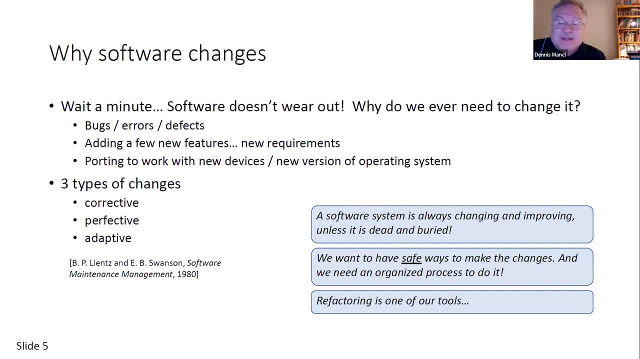 You know what's the new tax formula going to be? Yeah, we didn't know, right. Sometimes we have to make changes in order to port something to work in a new operating system right Now. have you ever used an old cell phone app and it doesn't work. It crashes. Well. 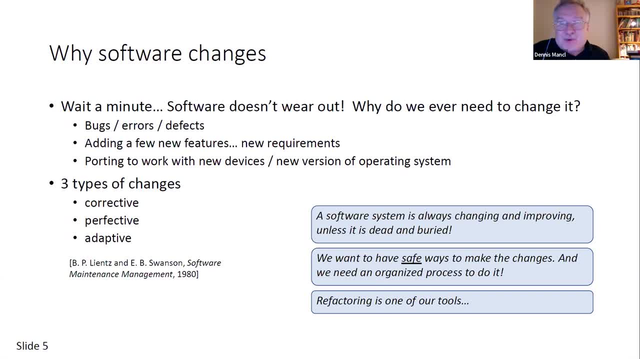 did you load a new version of the app? Did you load a new version of the app? Did you load a new version of iOS on your iPhone or a new version of Android on your Android phone? Yeah, that might be the root cause. So yeah, We really have three different kinds of changes. 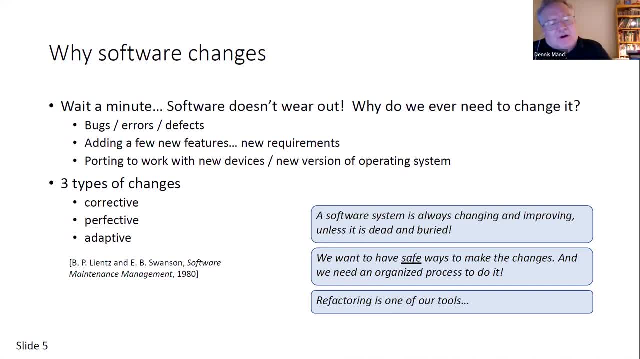 and we've known this for a while. I'm quoting here Linson Swanson in their book on software maintenance from 1980.. And they said: hey, there are three different kinds of changes that have to happen in our software. There's corrective changes, like the bug fixes. There's perfective. 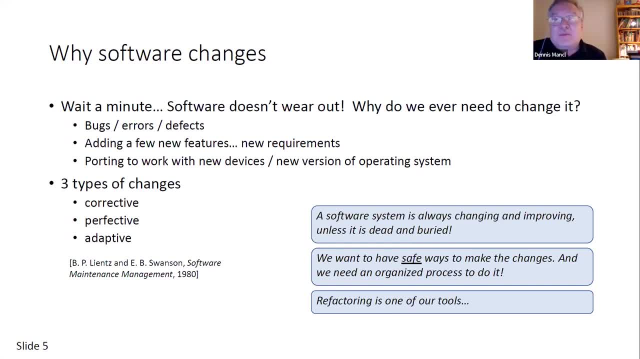 changes, which are? you know, we've got, you know, new requirements that are coming in. And then there are adaptive changes like those. oh, you know, somebody upgraded the operating system. We'd better fix our application so that it can use it. Yeah, The only time an application. 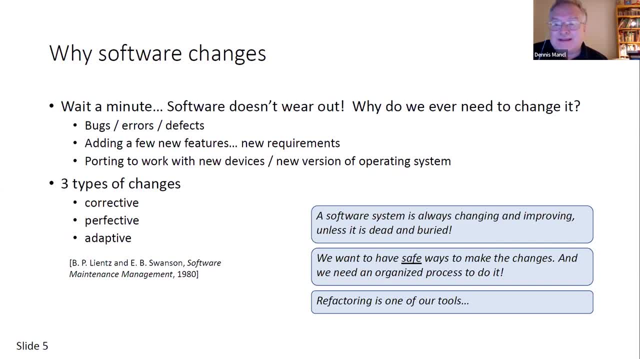 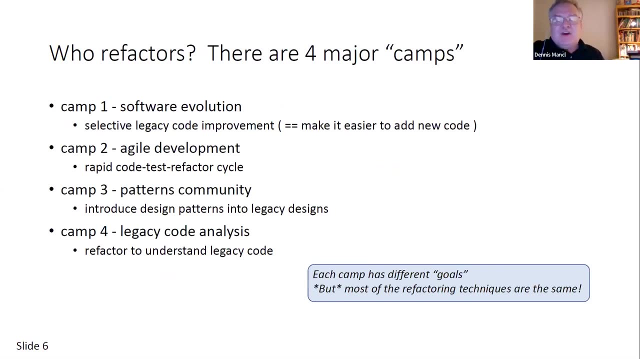 stops changing is when it's dead- right Dead and buried. So how do we think about making changes And how do we think about refactoring? We want to make changes safer. So it turns out there are three really important slides in this presentation, And you can tell they're important. 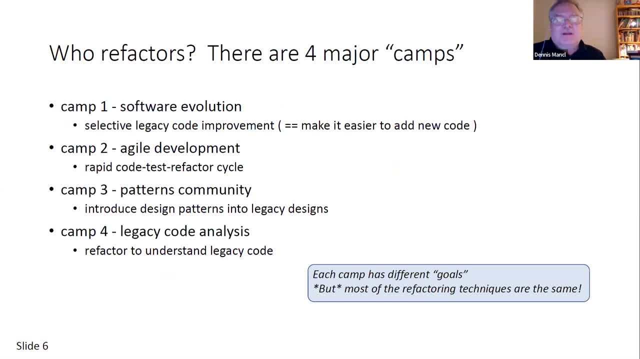 because they have a little star up here in the corner right. The star says: hey, remember this. So refactoring doesn't necessarily have the same meaning to everybody. There's really four different camps. There's the software evolution camp, There's the agile development. 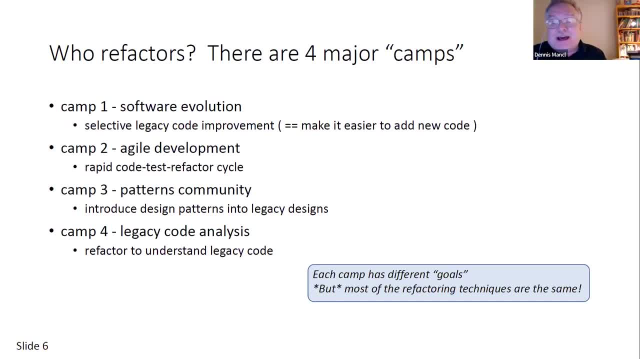 camp, There's the patterns camp And there's the legacy code analysis camp. We're going to talk about all four of these in this talk right. Camp one is focused on the evolution of your application, Like my telecom friends, you know, would have this problem. Camp two: the focus is: 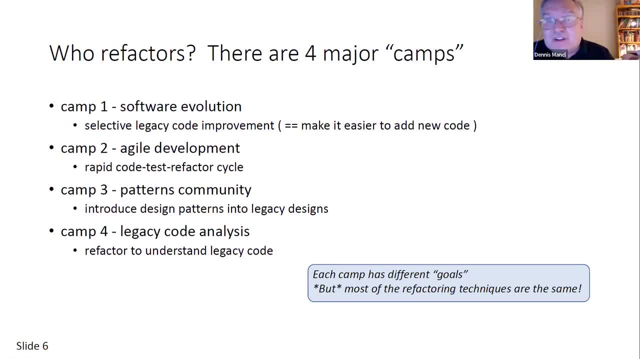 on being agile, working in short iterative cycles. Camp three: we're expanding beyond just simple code changes. We're expanding beyond just simple code changes. We're expanding beyond just simple code changes And we're looking at improvements in design, applying software patterns And camp. 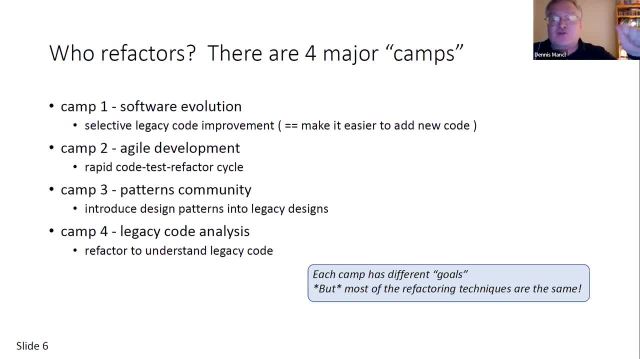 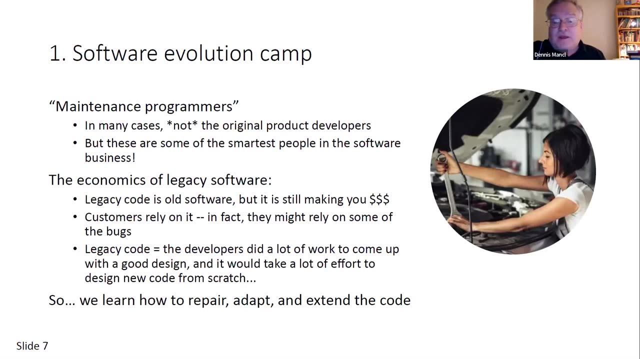 four is all about how we can use refactoring as a tool to help understand old code. So each group is trying to do something different, but it's still called refactoring. So consider the fact that refactoring may have different goals. Okay, So the software evolution camp is home. 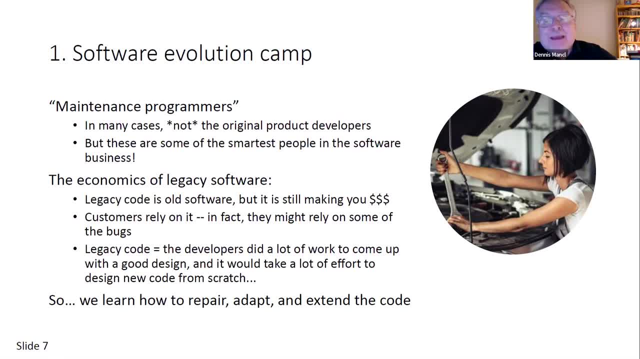 turf for the folks we call maintenance programmers. Now, maintenance programmers are some of my favorite people, right, It's my favorite people because they're really smart. right, They open up the hood right of existing code and they know the best ways to go in and fix and extend. 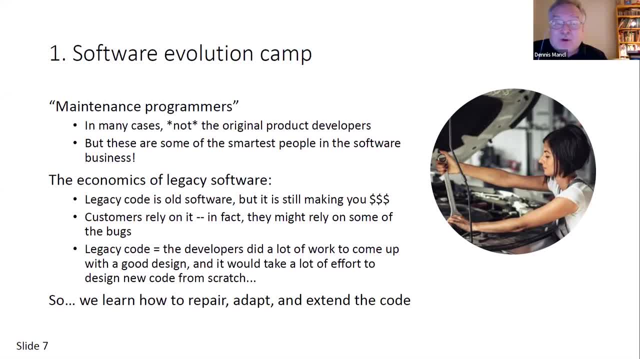 the code, Legacy code, right, Old code that you know, somebody you know wrote and you know they're gone and you know now they've been abandoned. Legacy code is not a dirty word to them, Because legacy code is code that makes money for the company. still, It would take an enormous 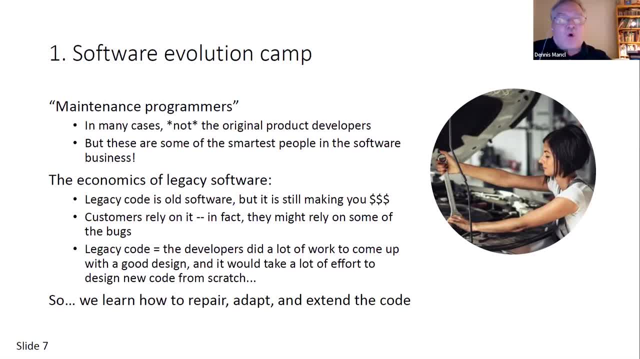 amount of effort to build a new system, with all of the expertise that went into building it. So, hey, repair and extending code is definitely something that's worth the effort, And in doing so, we're expanding beyond just simple code changes. We're expanding beyond just simple code changes. So 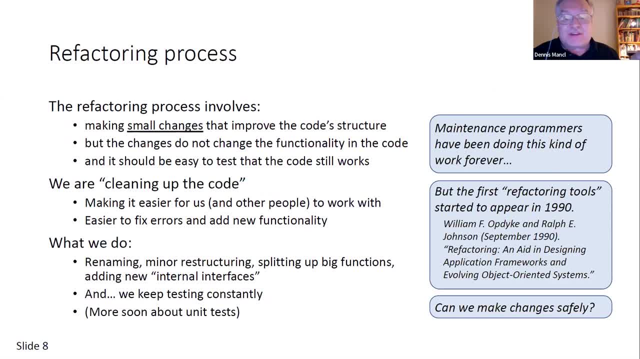 and in doing maintenance programming. refactoring is the process of making selective, small changes. you can see right and testing to make sure that things still work. So when you're refactoring you're not a hacker. Hackers aggressively blow up code. Maintenance programmers change things. 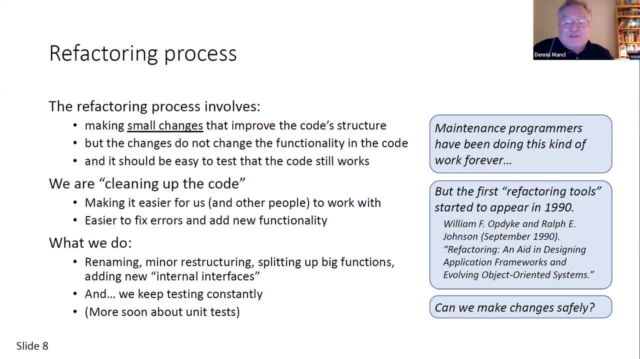 slowly and well. When you spot a bug, you may say, oh, I'm going to gently improve the code around it with some refactoring, All the while testing to make sure that the functionality is still the same. And then, when I fix it, I say, oh, okay, now I'll make a one or 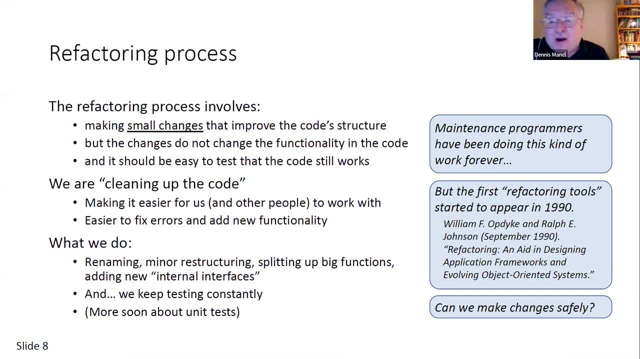 two line change And, yeah, that's just going to fix the problem that I'm trying to fix the bug for. So the refactoring work is the preparation to make the fix simple and to make sure that it stays fixed, And we may actually do some other selective code improvements. 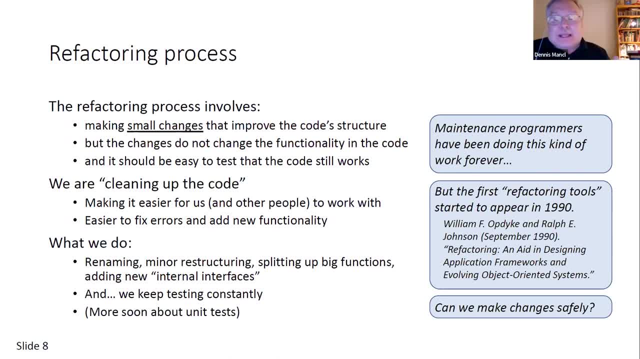 Like renaming, minor restructuring, splitting, adding internal interfaces. Now, this is actually the kind of work that maintenance programmers have been doing forever. Right, But the first refactoring tools actually started appearing in 1990.. And it was my old friend, Bill Updike. Bill worked for Bell Labs in Illinois. 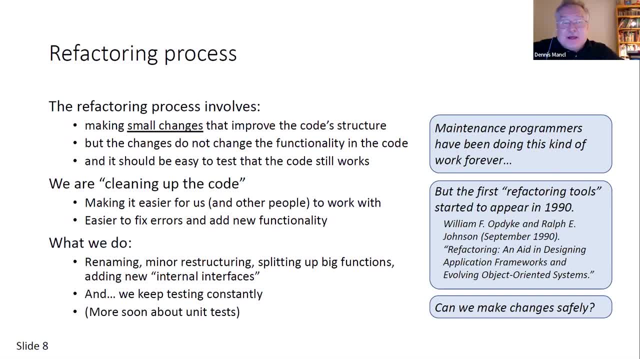 And he actually left the labs and went back to University of Illinois for his doctorate degree And he did a series of papers with Ralph Johnson, one of the patterns guys, And he did his dissertation on a set of refactoring tools And other people picked up on the idea. 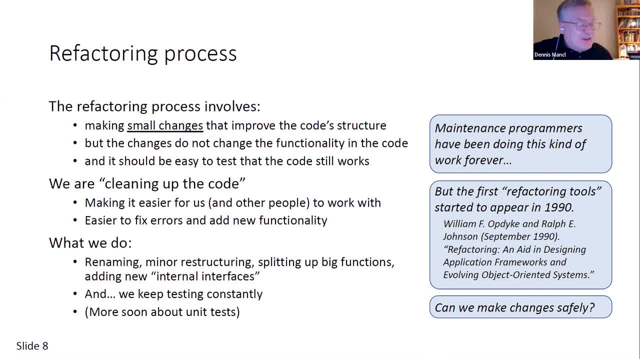 And they said, oh, we're going to put refactoring into some of our code browsers and code editors and stuff like that. And from that point on, this idea started to gain some motivation. This idea of making changes safely got a name. 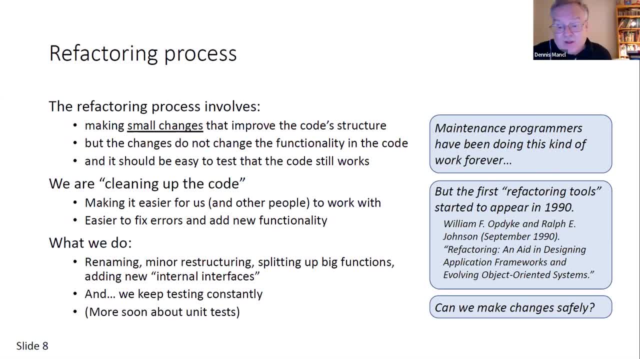 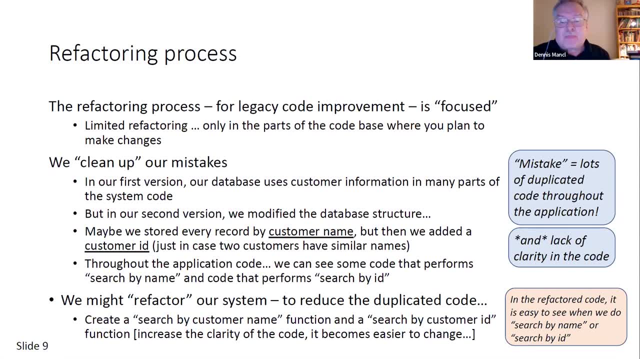 It became known as refactoring. So in refactoring in camp one, it's focused. It's focused. You refactor only where you plan to make changes soon. You're going to want to make sure that the code is clear and understandable before you make the fixes. 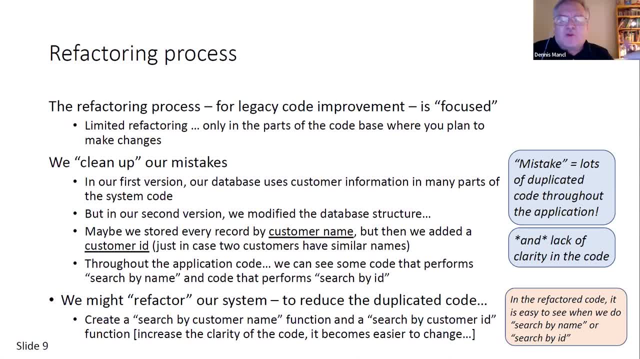 Thinking of it as fixing our mistakes. So, for example, you might have a system that's doing all kinds of ordering and shipping products, where your database runs on customer name, But somewhere along the line you said, oh, we're actually going to add a customer ID. 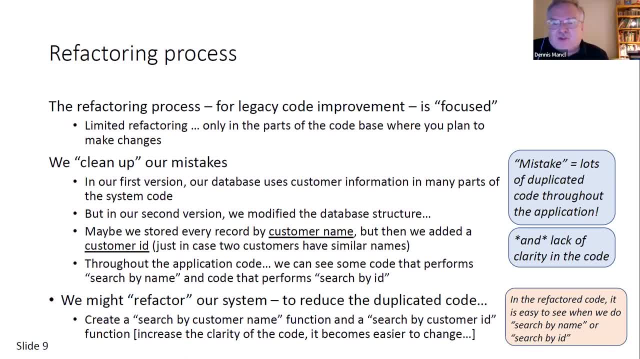 And the customer ID is an extra field that just makes sure that the customer information is unique. But all around the system there's a system you have searches on customer name, Or is it customer ID? I don't know, It's a mess. 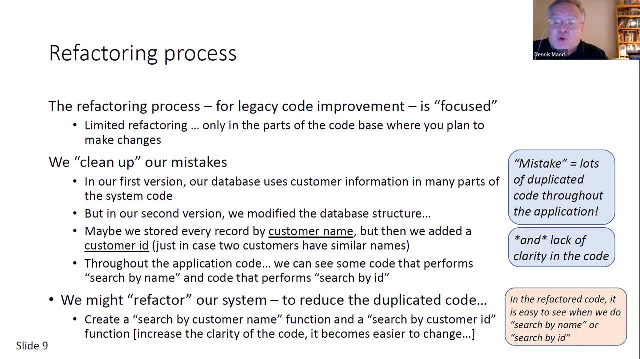 You're looking through the code and you can't tell. So what we do is we say: let's back up, We're going to refactor slowly to create search by customer name functions and search by customer ID functions, clearly labeled, And then slowly replace the code which. 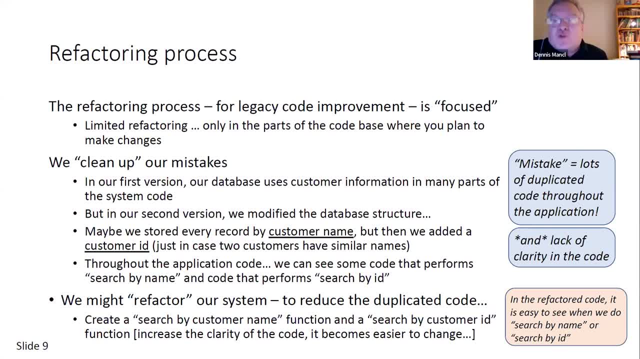 has lots of ad hoc queries all the way through it to use those new new functions that we extract so that it's clear at a glance. We look at this code and we say, oh, that is the kind of search that's actually taking place here. 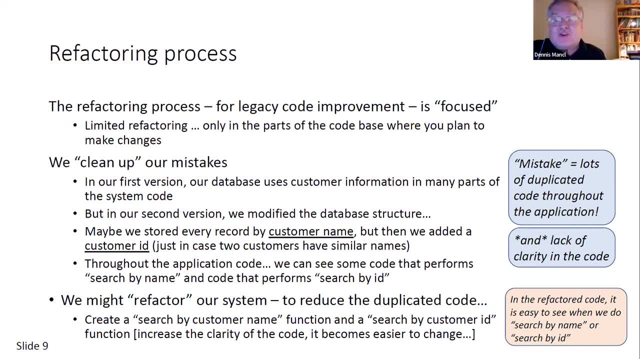 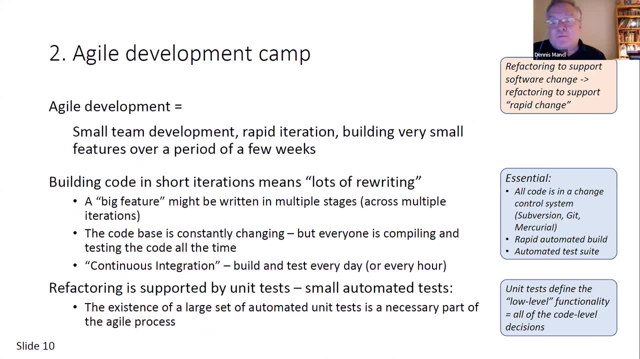 So yeah, that's the kind of clarification that happens all the time in refactoring. Now, camp two, We're going to talk about agile developers and agile development. Agile is really a movement Within the business of developing commercial software products that started in the mid-1990s. it became very popular. 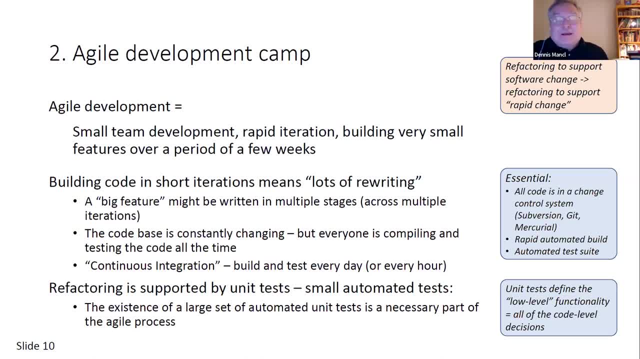 for developing web-based software, for building mobile apps, because you're building lots of things that are small and you need to get them done quick. The chief characteristics of agile development are small teams. Maybe you'll have 3 to 10 people on a team. 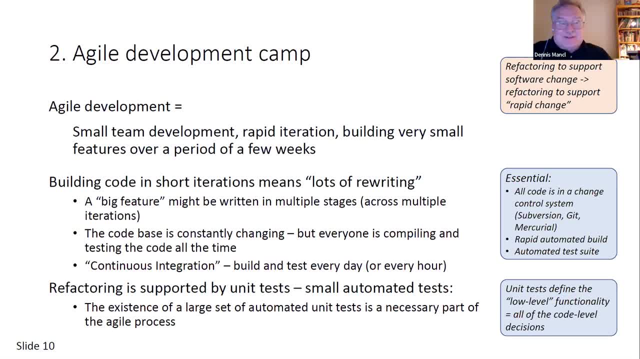 It's not our big Bell Labs AT&T, You know, 100-person, 180-person project- No small- And the team is building small features in a couple of weeks And they keep iterating to build a bigger product right. 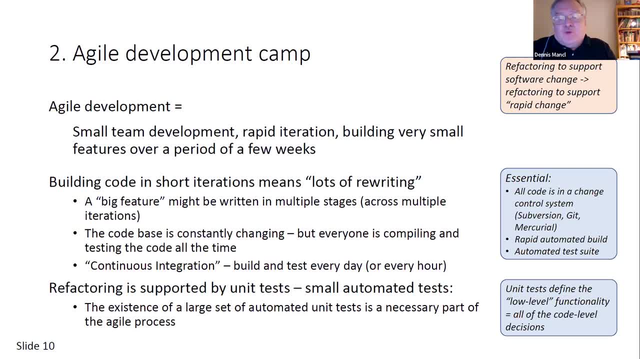 And, of course, they keep talking to the customers, because what they're doing is they're helping to set priorities. Which things do the customers want first, Which is most important to them, right? So what happens in this environment? and this is: 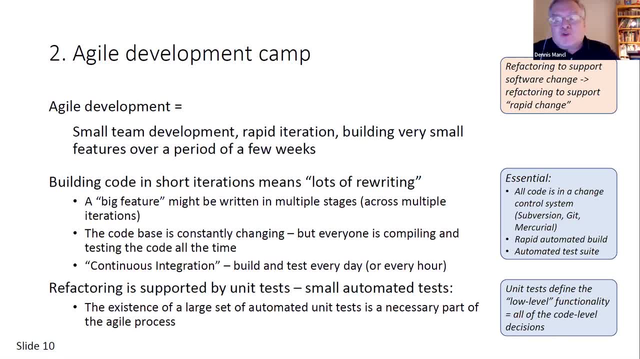 the second block. Here. any work that you do early will need to evolve. You'll have some rewriting done on it, right? Because you're always starting with a few small features and they're incomplete And you're expanding them to whatever. 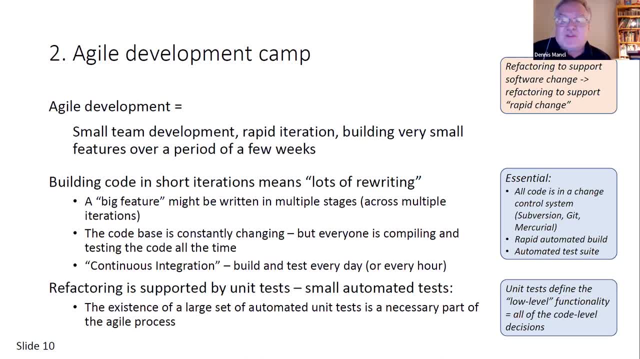 the customer really wants. So you might be changing course if the customers change their mind. Notice that agile developers use continuous integration to compile and check their work, frequently Fixing small problems, And agile development uses refactoring all the time, in every iteration. 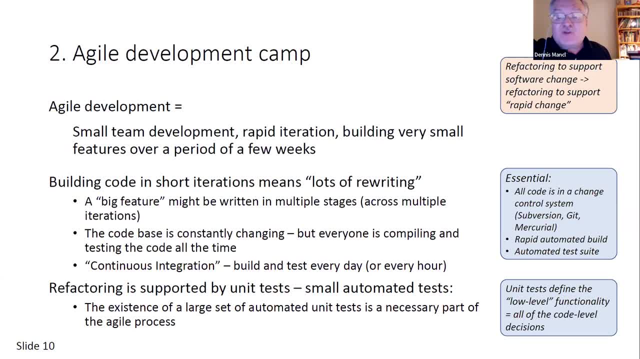 And frequent building and testing too. So this is where building unit tests gets to be important. It helps to support safer refactoring. By the way, as a side note, agile teams are in the habit of using a version control system or a change control system. for all of a sudden, 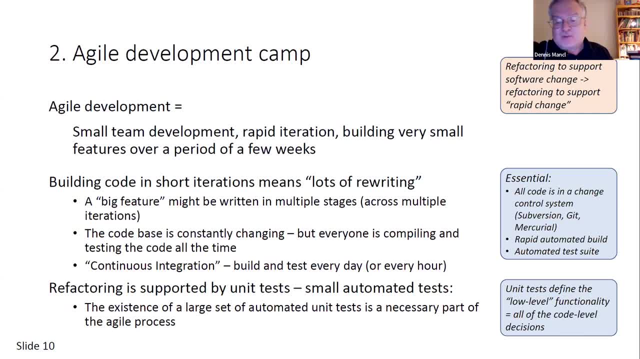 Right To build: automated support, automated build and automated testing. So you can see over here on the side, you might use Subversion, you might use Mercurial, you might use Get And all your code is kind of being checked in there. 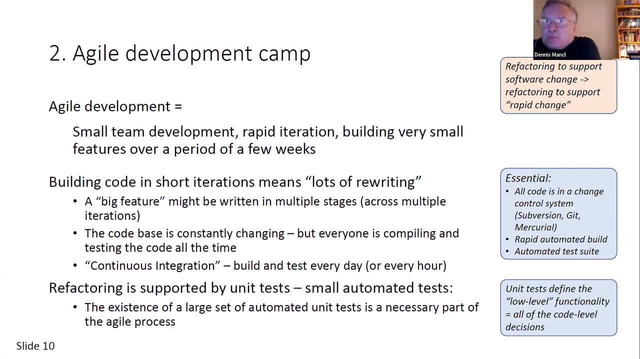 So you can always go back to a previous version. You can make a little branch and say, oh, I'll try this out over on the branch, and then merge it back in Right. So this change control is a big help in the step. 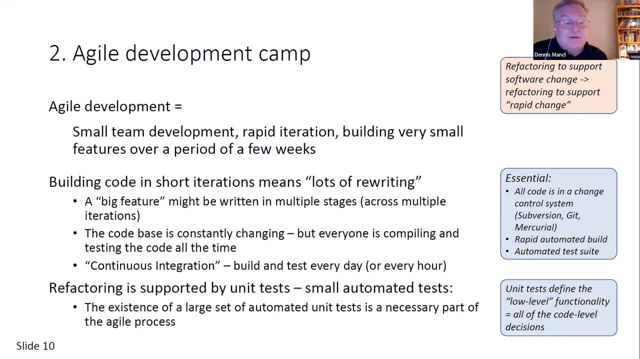 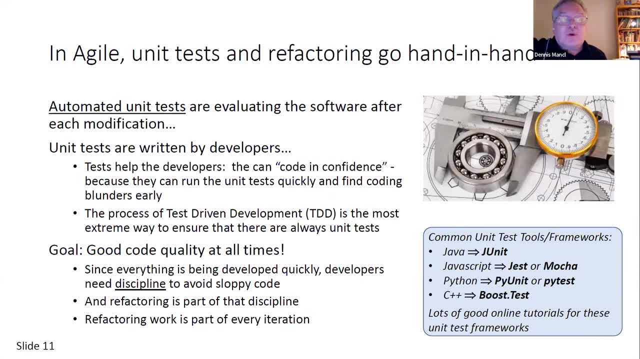 by step refactoring process. All right. So unit testing and refactoring go hand in hand, Evaluating software after each small change. you have an investment in unit tests. You'll see agile developers use test driven development. Test driven development is a little strange. 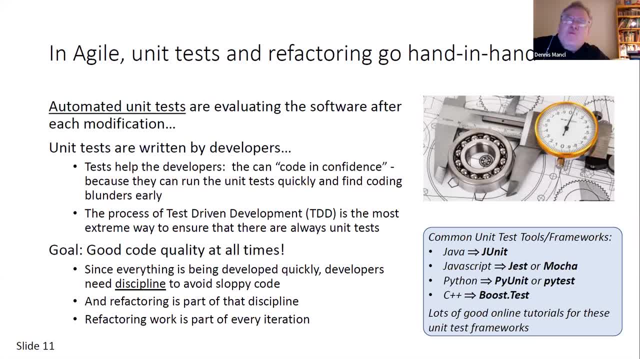 You're running some unit tests every few minutes while you're coding Right, You're making small changes to implement a new feature And you're developing the tests at the same time. In fact, what you do is you put in a test that you know is going to fail. 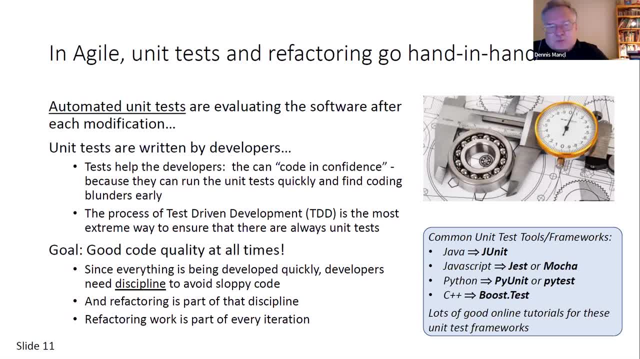 Right, But you want to have it succeed. They haven't written the code for it yet, So you put it in, You check to make sure that it actually does fail, And then you develop just enough code so that that test passes. And then, of course, you check all of the other tests. 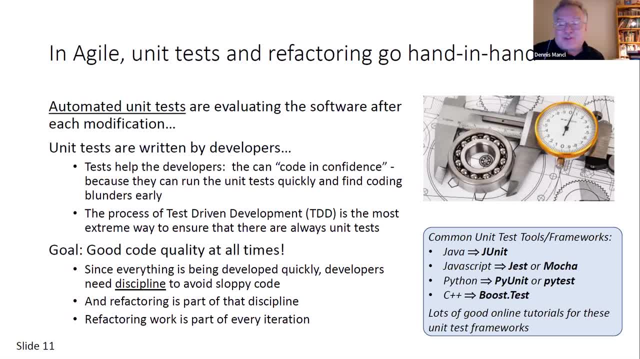 to make sure that you haven't inadvertently broken anything else. This test driven development is a common technique Right In these fast operating iterative agile development projects, And it's a good discipline. Without good tests, developers get sloppy. By the way, you might want to learn how to write unit tests. 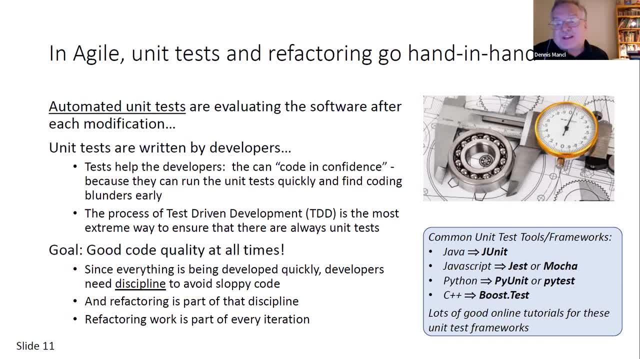 Right, Maybe with one of these unit test frameworks that I've indicated over here on the right Right: JUnit for Java, Jest for JavaScript right, PyUnit, maybe for Python Right. There's. many languages have these simple unit test frameworks. that makes it easy to plug in small tests. 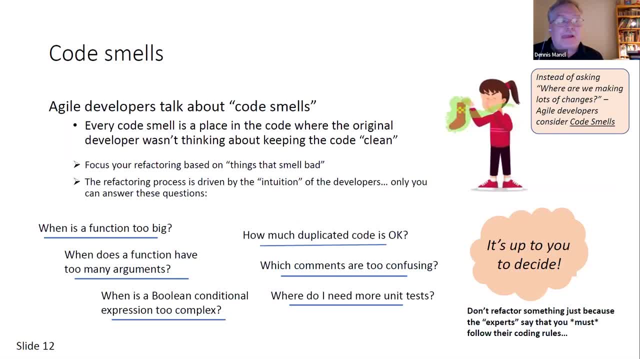 and have them run automatically. Cool, OK. So I said before: what's the strategy to decide what needs to be refactored? Well, in camp one you're thinking about what's going to change next. But you can't afford to do that in agile because, hey, next week. 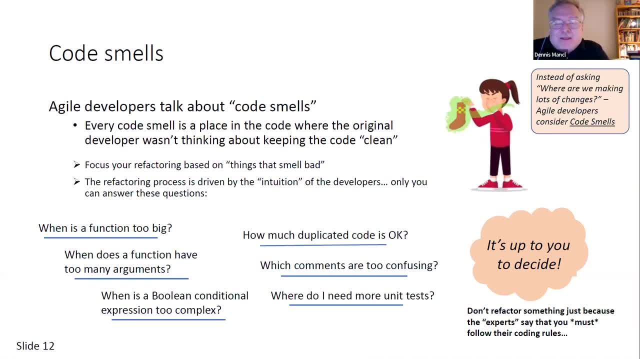 you may be working on something But you didn't think you'd be working on, OK. So in agile, what you tend to do is use code smells to determine which kinds of refactorings might actually be helpful. The code smells are standard code quality issues. 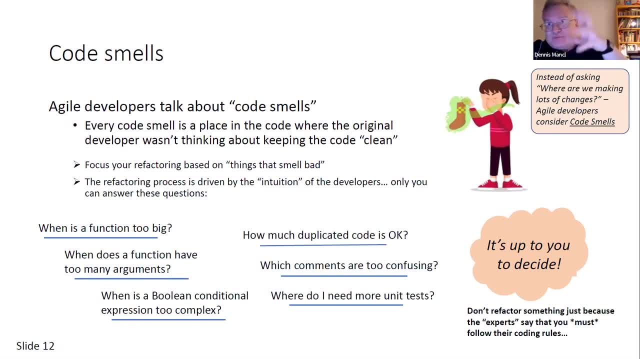 And you have various catalogs of code smells If you don't know them. You know You can find some of these things on the internet, But remember I said that there's a little star up in the corner of the slide. This is like something that's really, really important. 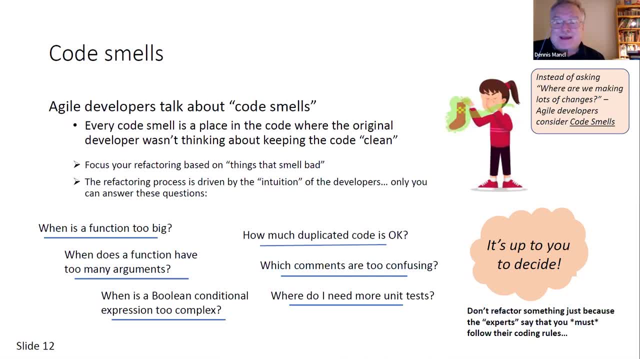 Well, guess what? This is really really important. OK, Use your judgment. OK, Somebody, some code smell, will say: oh well, large function, Large functions are bad. How large is large, Right? And Is This particular function an exception, right? 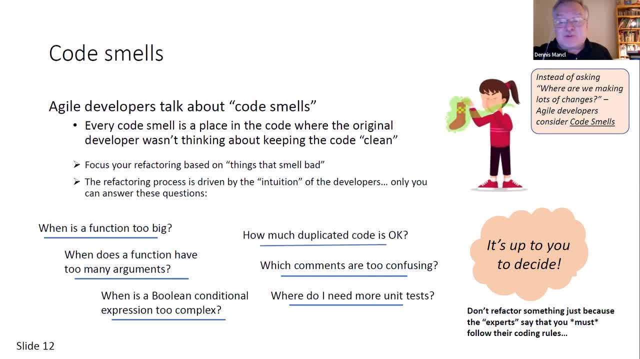 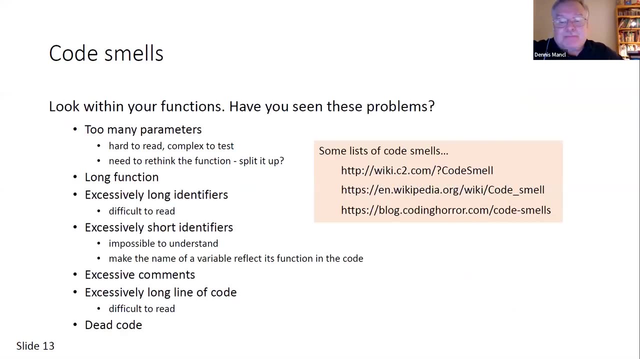 Don't refactor something just because the experts say that you must follow their coding rules, because you'll never finish. Your judgment should be your guide. It's your decision what you want to work on today, Cool. So here's some code. smells right. 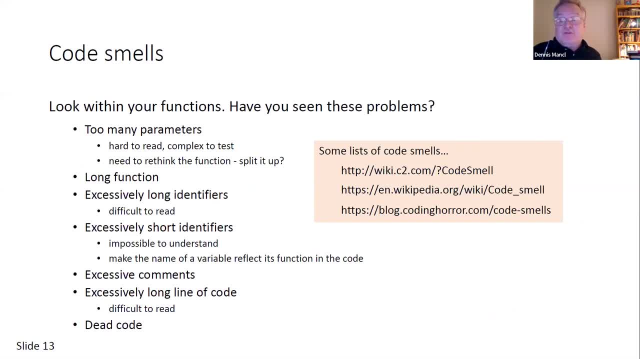 These are some of the function level code smells And, by the way, There's easy refactorings to go with each of the smells. In general, you'll see from these code smells They're often about length and or complexity that makes something smell not so good, right. 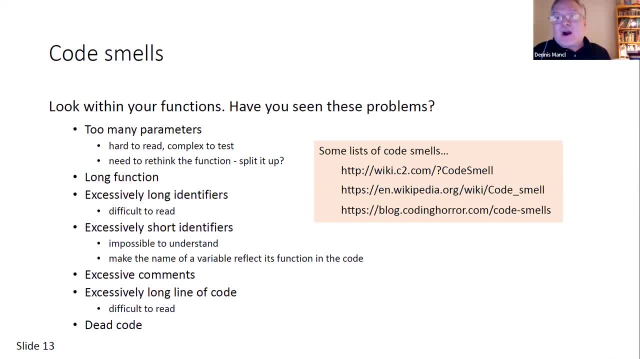 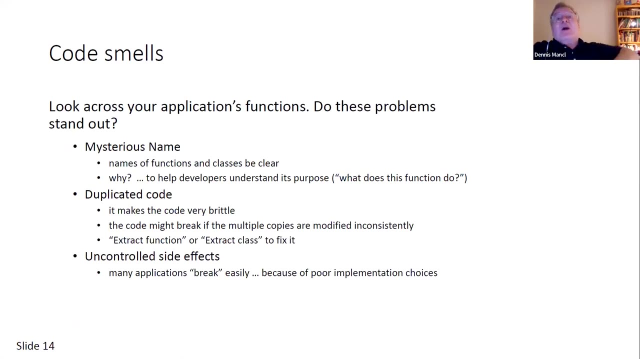 Too many parameters. long function right. Excessive comments: right. Comments should be short and sweet And they should always tell the truth. I wish All right. There are also code smells that apply across functions right? Or you might have to look in multiple source files. 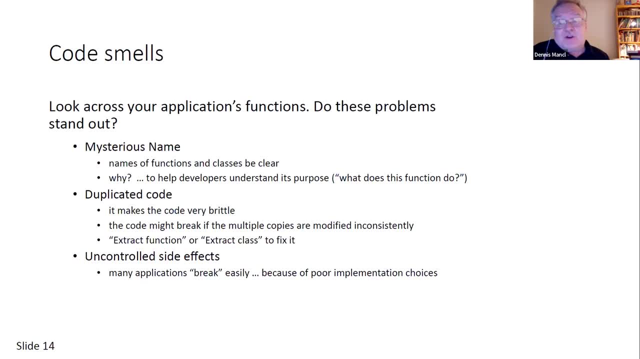 to trace down problems. For instance, you have a bunch of code where you're working over here and you're saying, oh, I'm calling this thing that's over here and the name is totally mysterious. You know it's a terrible name for a function, right? 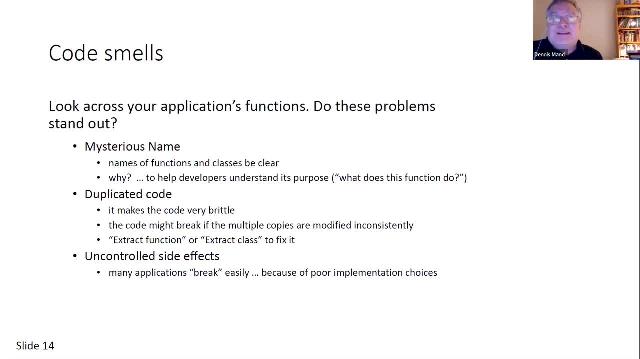 You should. The name should reflect Its purpose, right, And it's usually because the person who wrote it, they knew exactly what they were talking about, But the people who are working off on other parts of the system, they don't know. 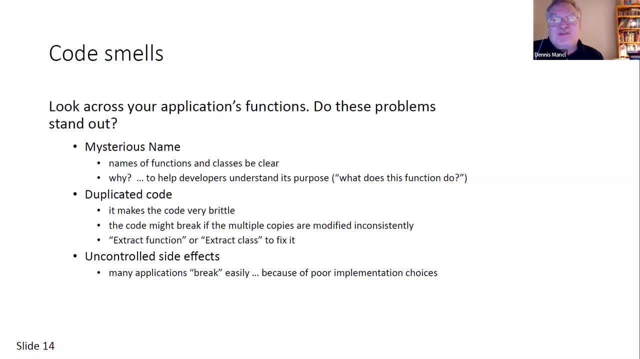 This could also cause you problems later on, when you actually look at code six months later and you say: what does this do? I've forgotten. Yeah, So good name helps, right, But duplicated code is another place where you have to look across multiple functions to find places where 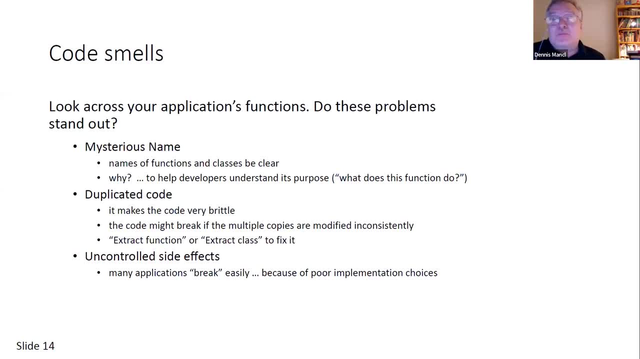 You're really doing the same thing Now. this actually makes your system brittle, because what will happen is somebody will find a bug right, And I say, oh, I'll fix it over here. Why I didn't get the duplicates? 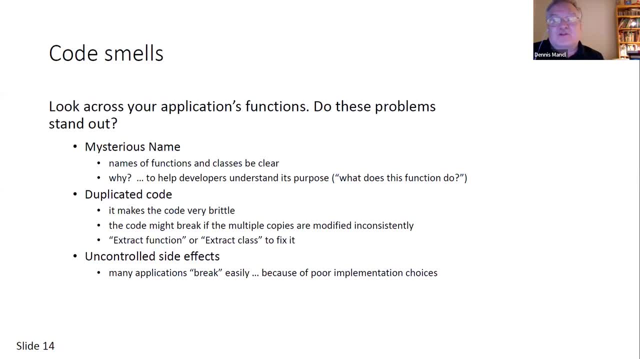 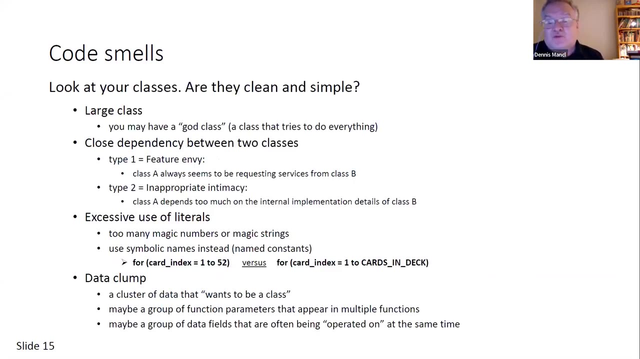 All right. So you'll use some of these refactorings like extract function, extract class to fix these kinds of duplications, And uncontrolled side effects are yet another problem that can happen, And it's often sloppy design that gets you there. Here's another list of code: smells. 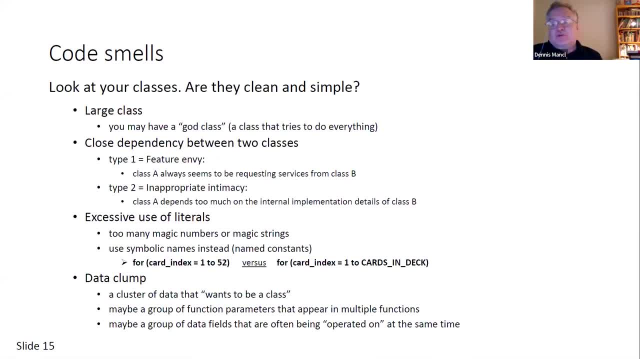 It's a lot of code smells that have to do with classes. right, If you're writing classes in your code, like in Java, Python, C++, JavaScript, big classes, what we call a God class- can get you into trouble and outside of the scope of today. 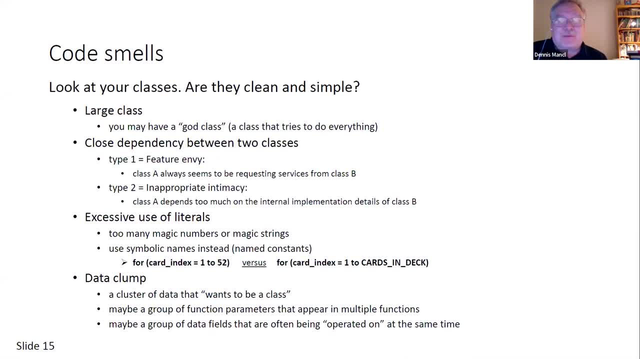 But meet me later if you really want to know how a God class can blow you up Dependencies between classes And I think there's really two different versions here. The feature envy of class A is always calling class B to do some work for it. 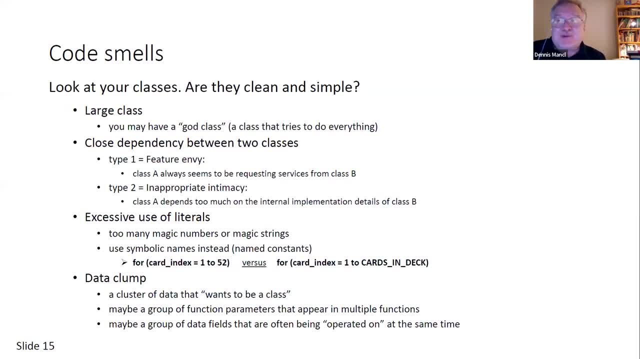 And it's doing it in a way that says class A says I wish I could do that myself And inappropriate intimacy is. the case of class A is far too dependent upon internal implementation details of class B. You really haven't written a good, strong interface for class B. 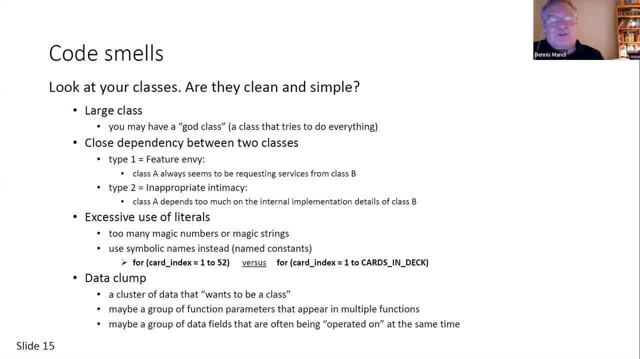 Magic numbers or magic strings, right? Here's some code where you're actually going through a List of something. Oh, they're cards in a deck of playing cards, because there's 52 of them. Well, use a symbolic name, Just don't use a number, right? 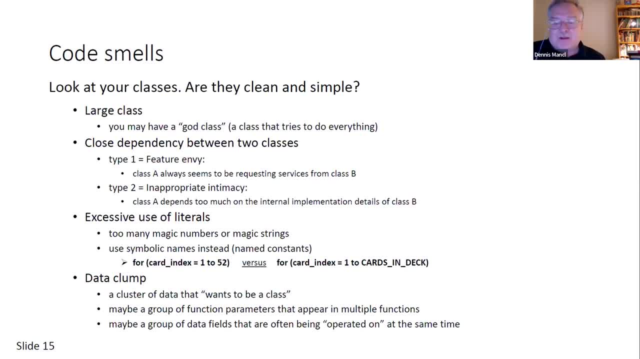 Cards in deck makes the intent much clearer. right, Data clump. It's a cluster of data that really wants to be a class, right? Maybe you have a repeated cluster of five inputs to a bunch of your functions or a group of five data elements? 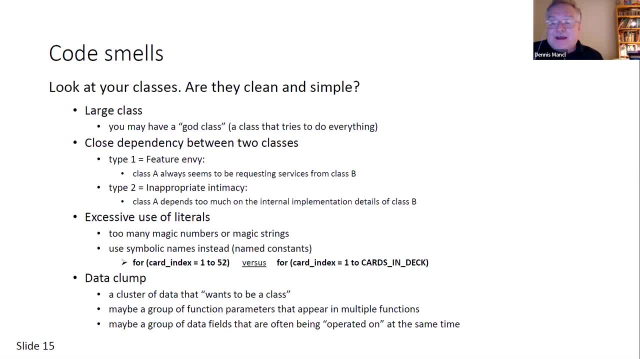 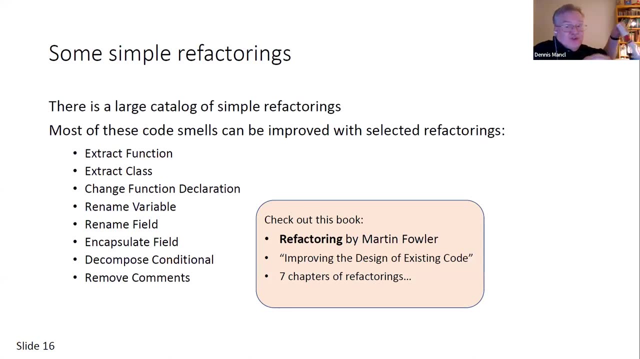 that are always being Operated on together, right, And maybe those five things should be bundled together and put them together into a structure or a class right, A record, something like that Class usually better. So I got to point you to my first book off the list here. 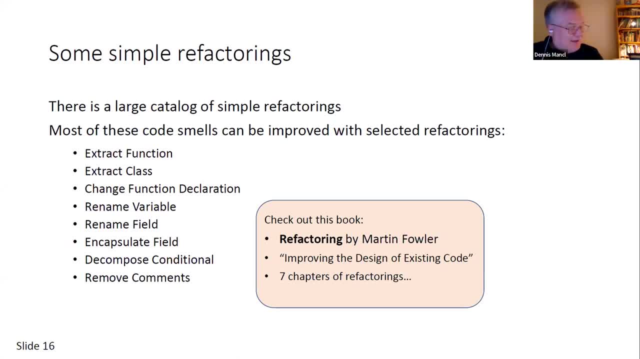 called Refactoring by Martin Fowler, And this kind of really got everybody going on this. Yes, Yes, Because what he did was he basically said: hey, here's some of the code smells, And here's some of the things we're actually doing. 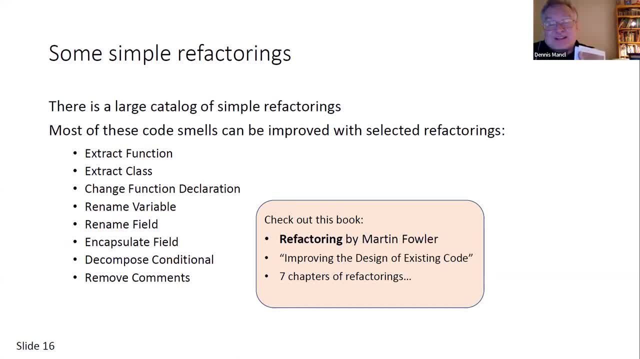 Now Fowler in writing. this book is very, very clearly in the Agile camp because he got a lot of help from this, from Kent Back, who's one of the creators of Extreme Programming, And so he's picking very, very small and actually very easy. 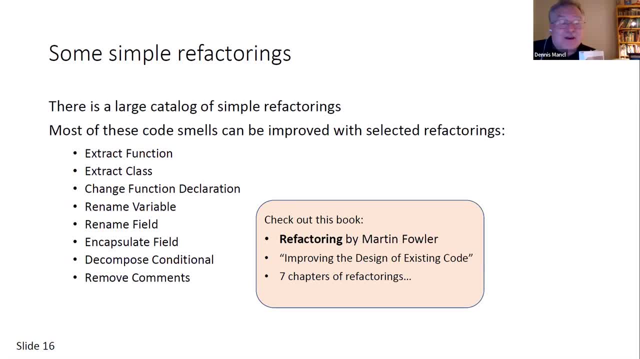 to do refactoring, But by having them in this catalog, it's really kind of cool. So I'm going to give you an example. They're all in JavaScript, But do they apply to other languages? Absolutely OK. Here's an example of a refactoring. 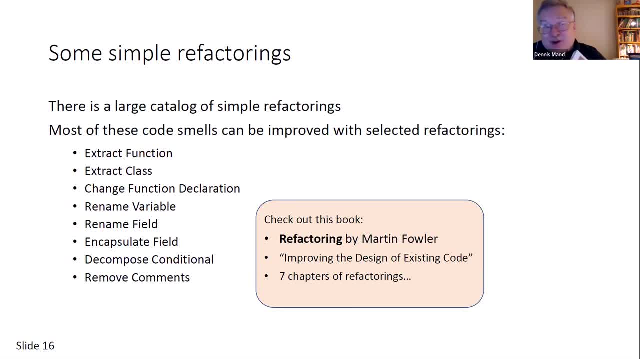 from Martin Fowler's book And I'm glad to be here today because I think it's a really interesting book And it's not just a piece of paper. It's a piece of paper that you can write with a pen and paper, But you can read it with a pen and paper. 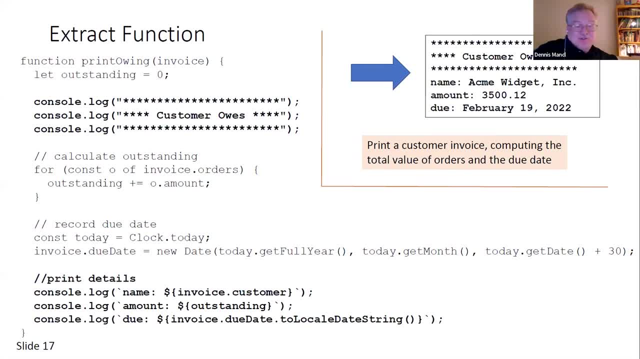 And you can write it in English. OK, grabbing the JavaScript version over here And here what you're doing is you're printing some kind of invoice right Here. you have up in the right hand corner, you can see it right. 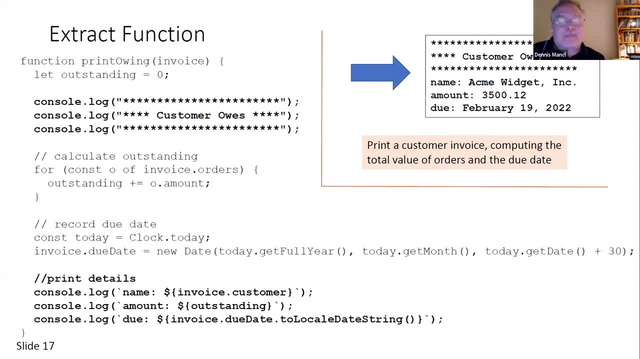 Customer rows and then name, amount and due. Okay, And you can see what it's doing is it's actually looping through a bunch of records inside this invoice object and adding those up and getting the billing date by just looking at today and saying: 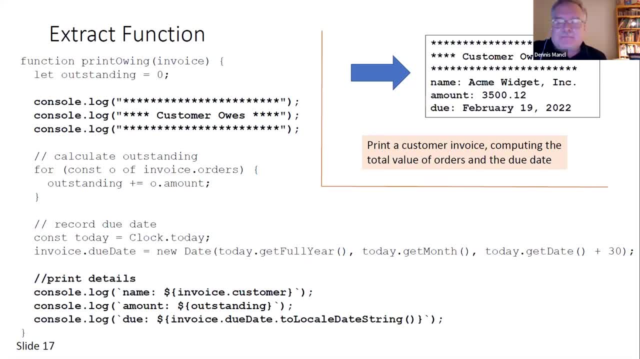 oh, let's go 30 days from now. Oh, that's where we're in: 18.. Okay, It's pretty straightforward in line code. Why would we want to refactor this? Well, one of the reasons is the output functions right. 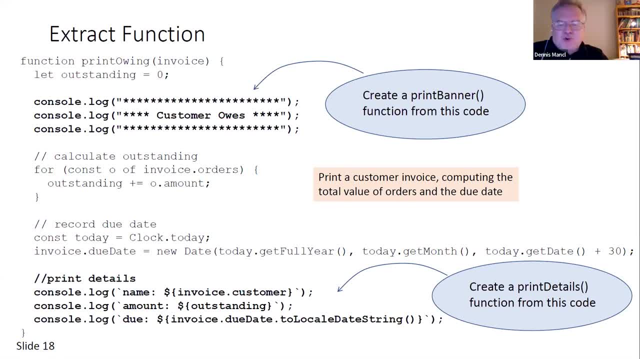 You're calling all of this stuff and say, hey, maybe we can push this down into lower level functions And we're gonna use the extract function refactor. It actually makes sense to me, right? Because the code that's printing the header might be changing independently of the structure. 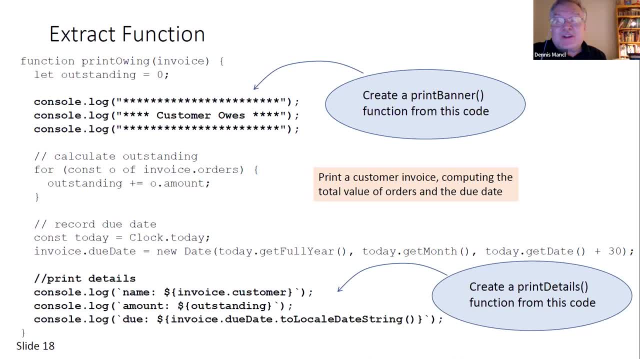 of the rest of the algorithm, right? So it's easier to handle that if this printing code, this formatting code, is isolated, So let's add those two print functions, right? I'm slurping those over and here they are in the orange boxes, right. 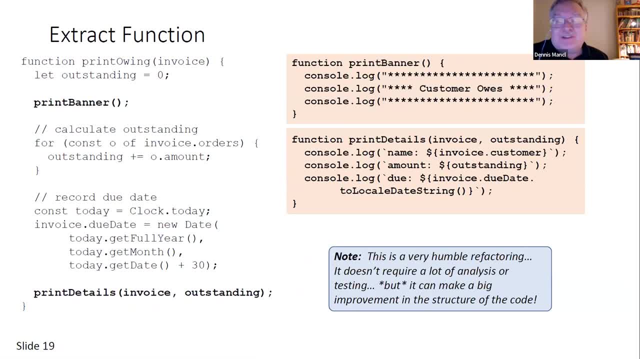 There's print banner, there's print details, very, I mean, trivially simple functions right, And now over in the main code, right, I just invoke them with the right arguments and you look at that code on the left and, yeah, that really looks simpler. 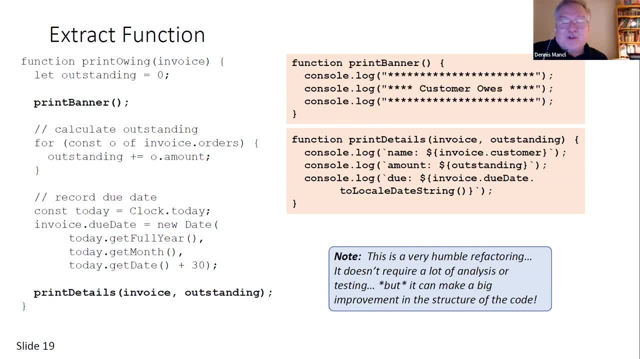 And it really does a good job of explaining kind of the flow of operations. It doesn't get messed up with all of that other garbage there because you put it into the lower level functions. Okay, Now, what we've done is just a very humble refactoring. 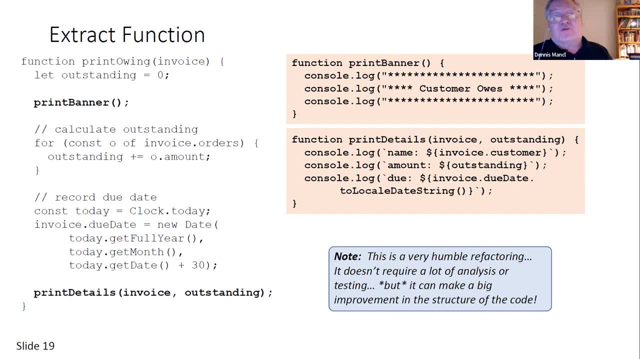 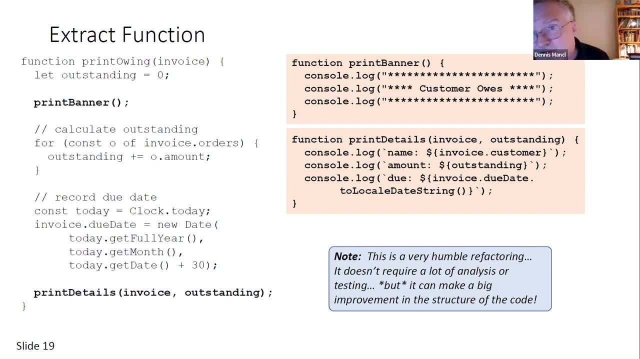 move many of the print functions into special classes. you know, yeah, And think about it. you know that would allow us to allow for different look and feel for different customers. We could say, oh, I'll have an online invoice. 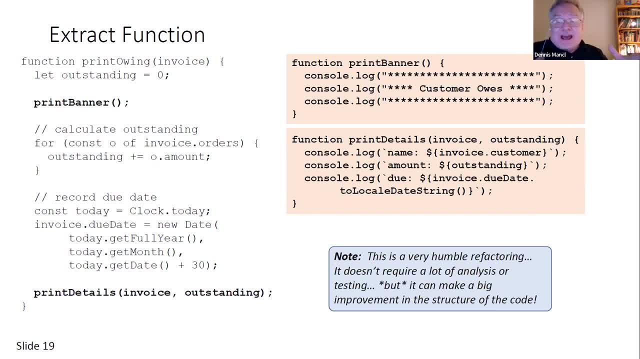 which we would do in HTML, of course- or we could have invoices that are separated out by subacademy Subaccounts, or maybe invoices in multiple languages. I mean, you're basically, once you start this refactoring stuff, you're actually paving the way by making the structure simpler. 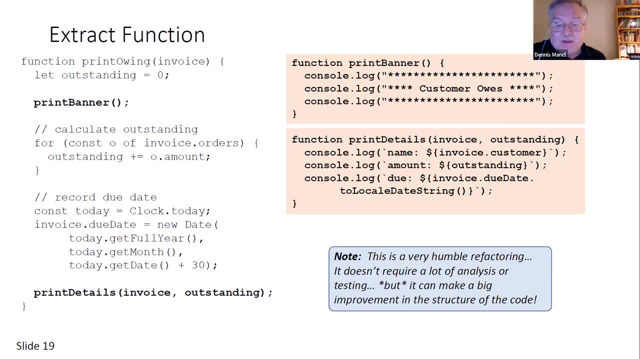 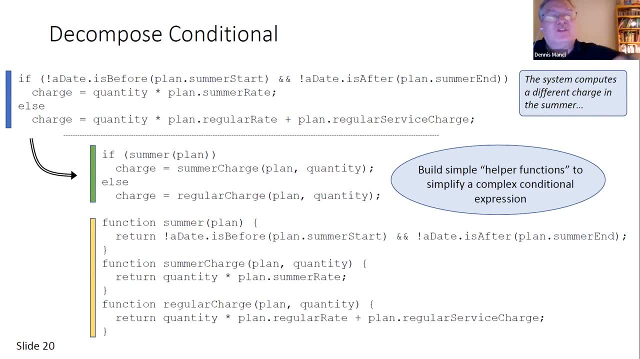 You say, oh, I've got some alternatives. Okay, Here's another refactoring, That's another really easy refactoring, And my original code's the one in blue up here, just these four lines, Right. And you say, oh, this is relatively simple. 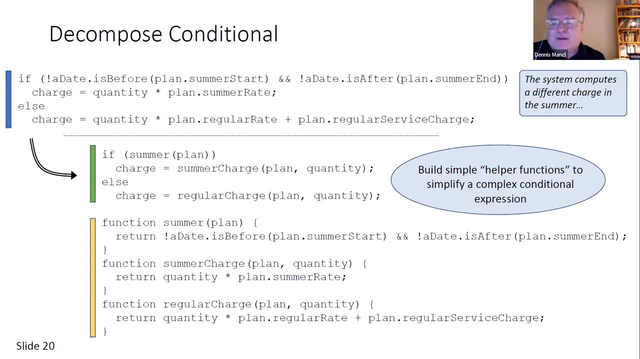 But it's painful because you can barely tell. right, it's almost almost obvious that there are two different computation algorithms actually going on in this code, right? Yeah, you're charging customers obviously different rates for, let me see, I guess, summer versus non-summer. 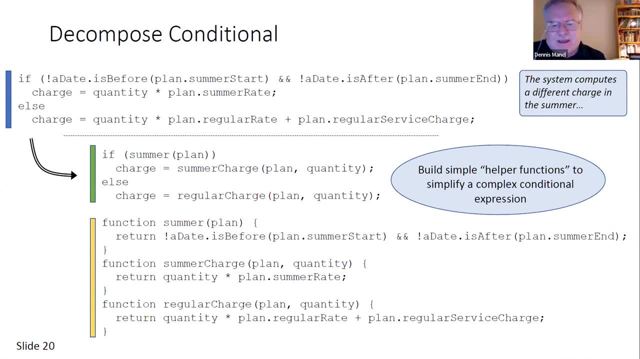 if I read this right, Any way that we could make this code easier to scan, right? How do we know if we got it right? Well, let's use the decomposed conditional refactoring, And then what we'll do is we'll extract out this conditional. 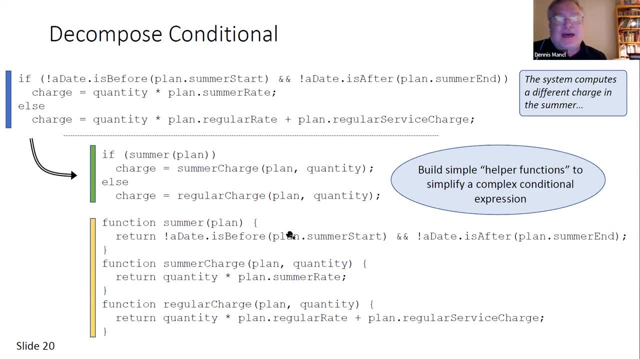 this big ugly is before and is after, and we'll just make it a function called summer, right, which has that conditional in it, And we'll just call summer in the green code here, right. And as long as we're doing that, well, 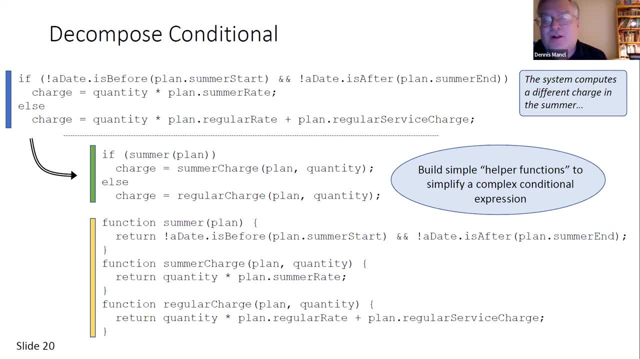 we'll extract the computation functions as well, right? So now our function is: it's still simple, It's still four lines, right? But we've pushed all of the really bad stuff into these helpers. OK, which I like, All right. 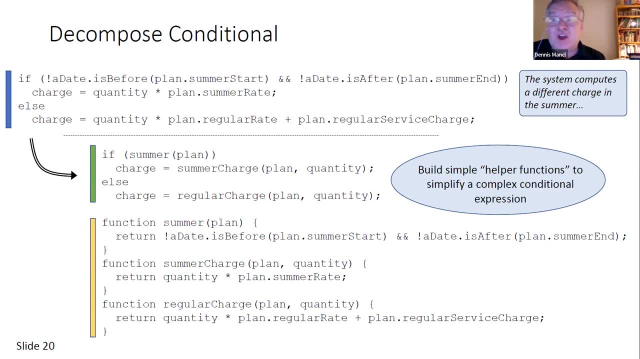 Did we save any lines of code? No, Did we increase clarity? You bet, And this could prepare the way for more right, Maybe a strategy approach for customer charging, more flexibility for adding other conditions, special discounts and so on. 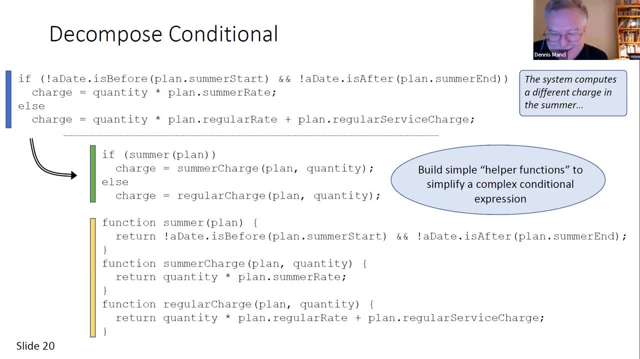 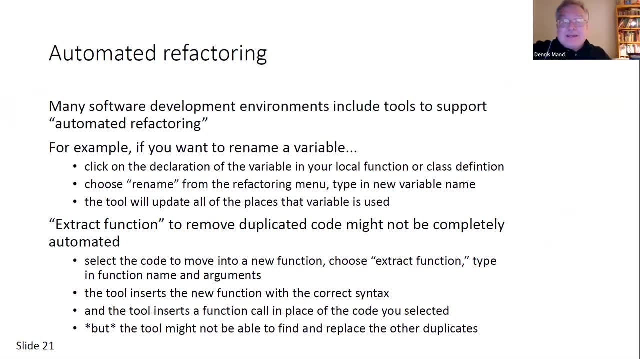 If you didn't understand that, don't worry. All right, Let's talk about automated refactoring. This can happen, right? You can say: I can use some tools to help me refactor, right? This is where all of this stuff got started, with Bill Opdyke. 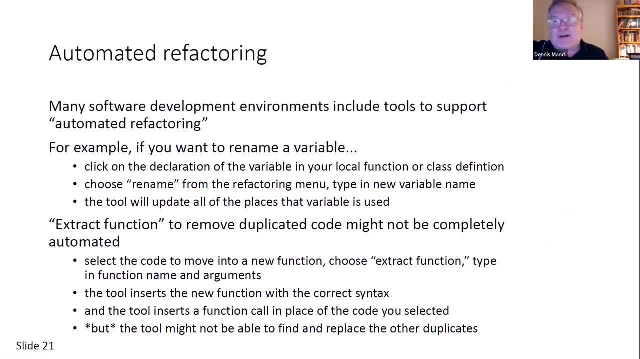 and people who were working in small talk And they said, hey, can we have some automated refactoring support for a relatively simple but powerful language? And I've got to say the tools can help right for things like: oh, I'm going to name my code. 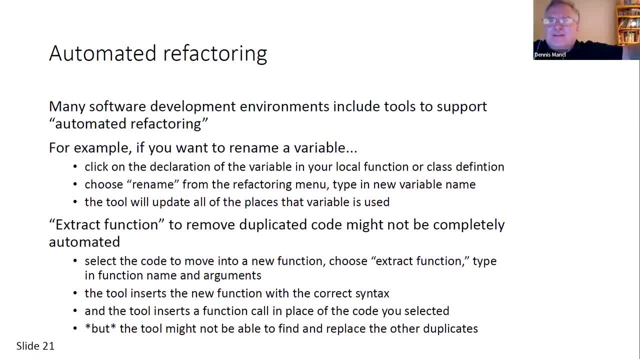 I'm going to name it in a different way. I'm going to name it in a different way. You can do some click right, Rename variable right, And you do some clicking And you're clicking on the declaration And it says: oh, I will find all of the uses. 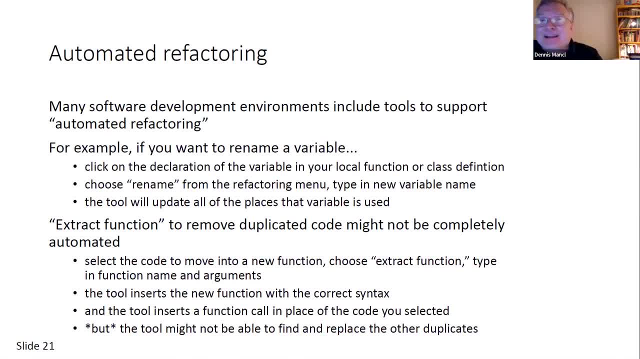 If you have an integrated development environment, it has all that in the database And it will rewrite everything right. Same thing with extract function. You say, oh, I'm going to highlight these eight lines of code And I want that to be put off into a separate function. 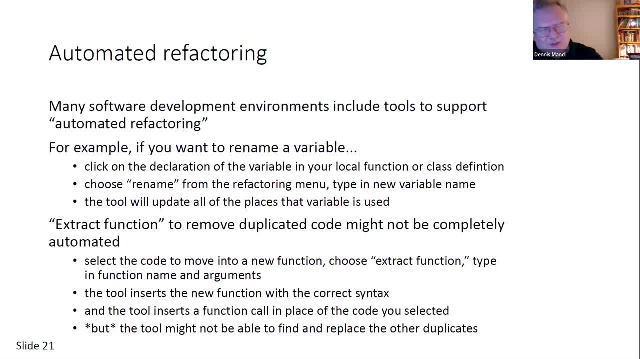 And then maybe, if it's a good tool, it'll scan through the rest of the code base and say, is there anybody else who's using the same lines? And it'll try. Maybe it can succeed and maybe it'll fail. 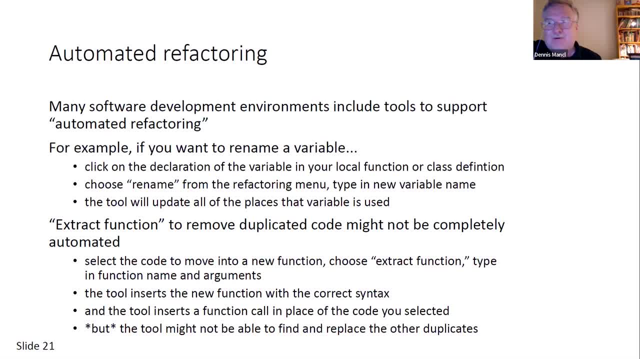 But it'll try to get all of the duplicates in there. OK, There's a difference between automated refactoring and automatic refactoring, And this is one of the places where, if you're a manager, it's easy to get confused. You say, oh, automatic refactoring. 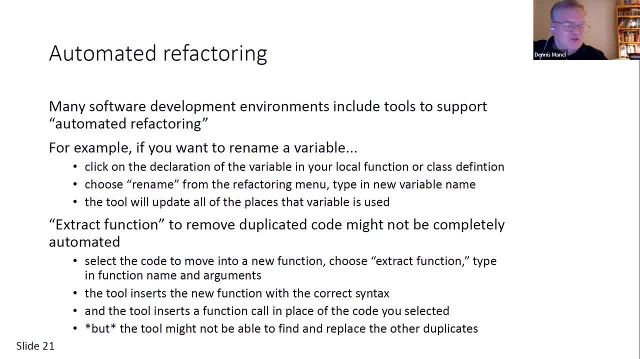 That's what I want. I want to buy the tool that I can just shove my developers aside. I'm going to shovel in the code, I'm going to turn the crank And out is going to come better refactored code. No, no, forget it right. 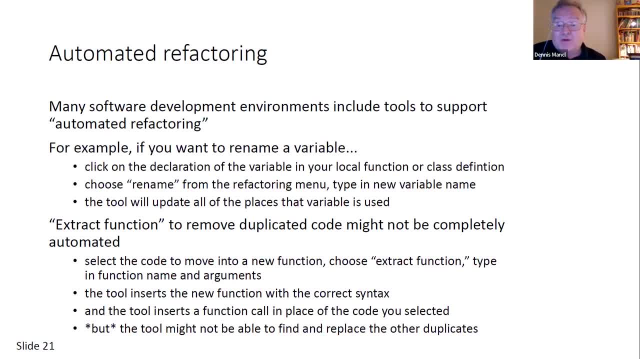 Because the tool doesn't select what to refactor You do right. You have to think about what you need to refactor, right, And that finding all the duplicate stuff is actually going to require some kind of experienced developer to go through and say, oh, this looks a lot like that. 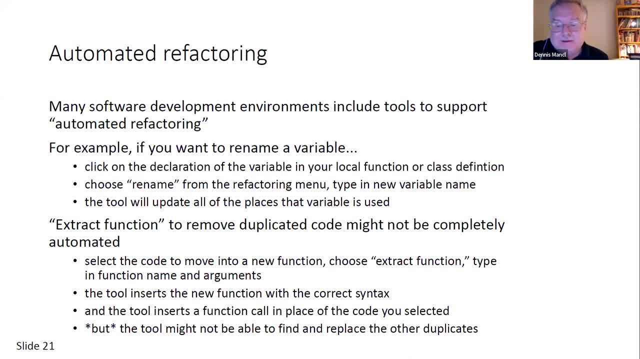 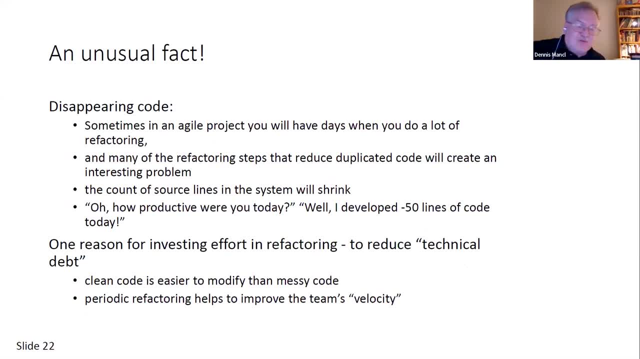 Let's see if we can fit that in All right. So something cool happens when you start refactoring- And this has long been something that's interesting, especially in this agile world that we're talking about- What happens when you start eliminating a lot of duplicates? 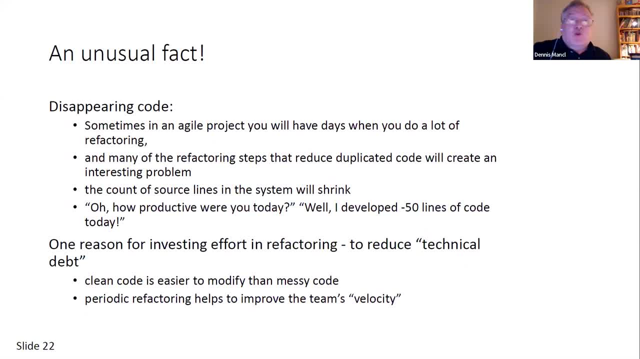 and dead code. OK, Well, you will have days, right? Let's say your team says we're going to spend Wednesday doing refactoring or Wednesday morning doing refactoring, And you plow through and you say, oh, I'm going to change this. 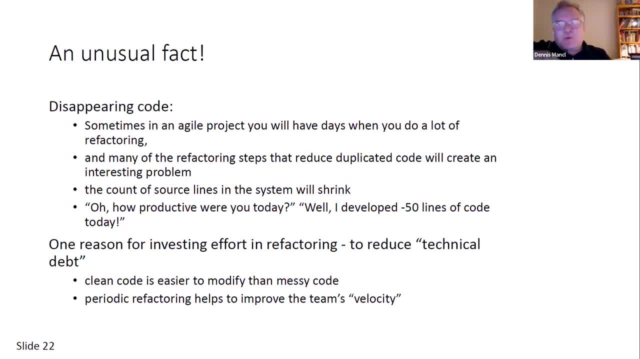 Oh, here's some dead code That's gone. Here's some places where I want to eliminate some duplication, And the count of lines of code in your code base has now shrunk. Now, as is inevitable, my boss comes along. 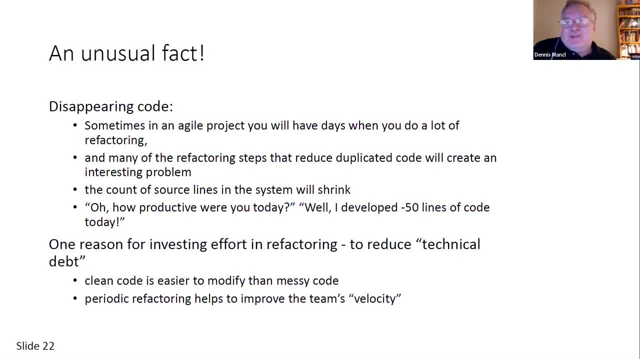 And she says: how productive were you today? And I have to tell her: well, I developed negative 50 lines of code today. And fortunately she's very smart And she says: oh, this is going to reduce our maintenance cost. 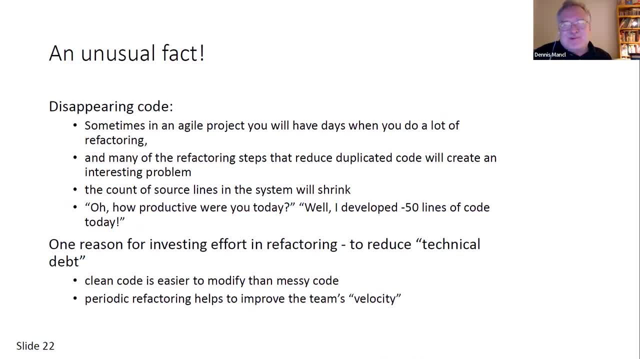 I said thank you, Because most people would look at this as a loss, But it's actually a gain, right, Because you're making simplification. You're also, by making that simplification you're making you're making it possible to add new stuff to the code. 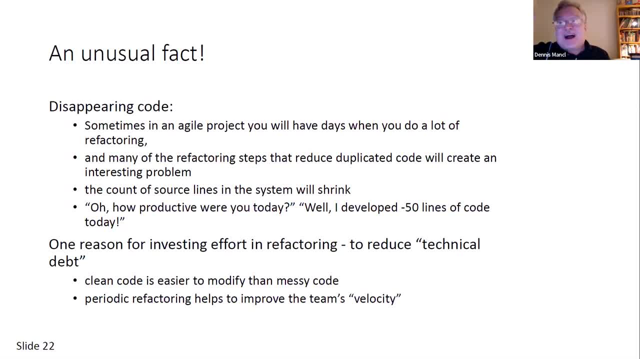 later on easier Because you're not going to be misled by things that are really clunky things in the code. I mean it's out of the scope of this talk to get into talking about it, But I will mention the word technical debt. 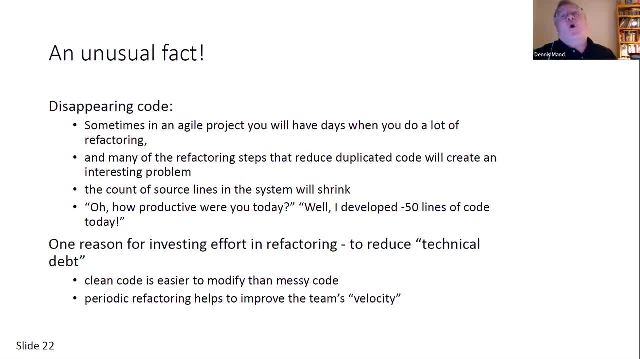 which is basically, you do something clunky and you really owe it to the code to go back and clean it up, But you often you're in too much of a hurry so you don't do it. Yeah, That's like a whole other talk. 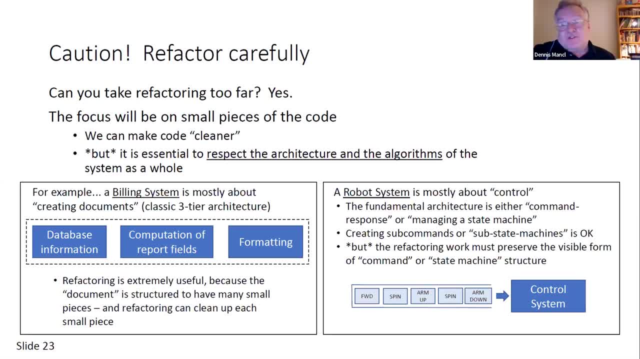 All right, Here's the third important slide. And the third important slide is- and don't panic about this one, because you will almost certainly get this right, or at least eventually- You may take a number of small refactoring steps, But then, as you work along, you're. 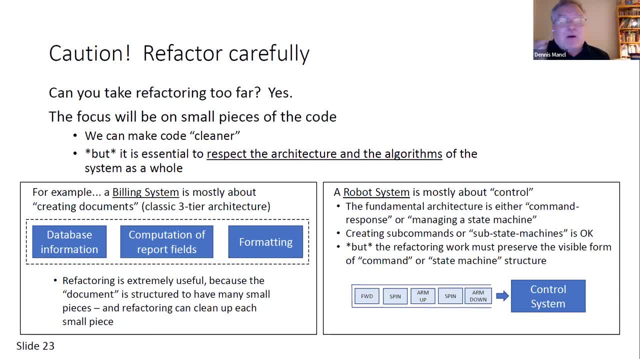 making your small changes, you could raise some problems. What I point out is that, refactoring, it's essential to preserve the architecture and the algorithms of your original code, Because, in some ways, these are fundamental to the way that your system works. 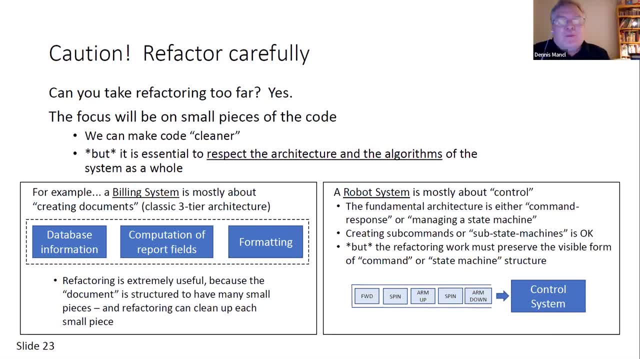 And as you're making individual changes, you may not see that, hey, you're wrecking the architecture of the system. In other words, you could blow it, But don't fret. Don't fret, And I'll explain why. Here's an example over here on the left. 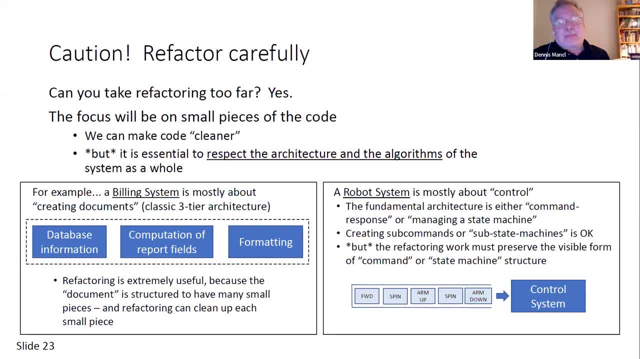 The left. here's an example. You have a billing system. Now, a billing system is really about the creation of different kinds of documents from a database and from certain algorithms and rules to compute the document's content, And in many ways it's a classic three-tier architecture. 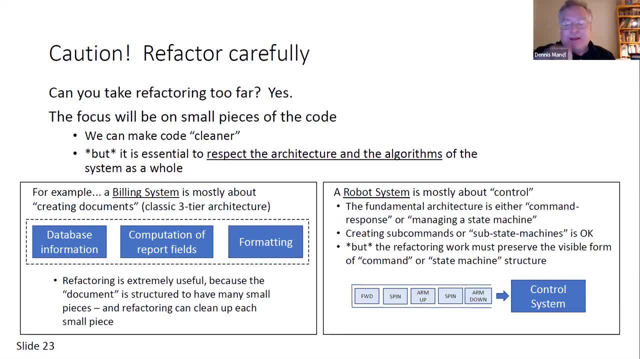 problem When you refactor code that's been set up in this billing system. you're going to do fine, Because most of the changes will be within one of the three big boxes: restructuring a couple of data fields, making an algorithm easier to understand. 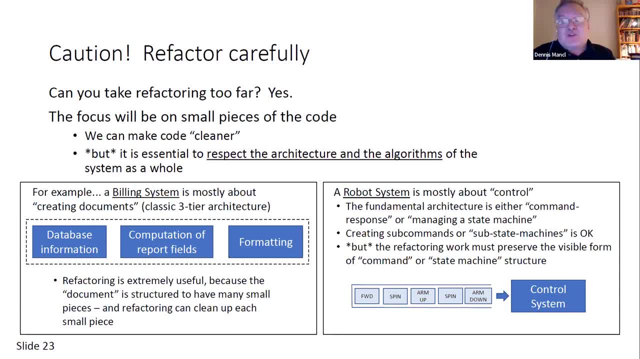 You're not really going to wipe out too much, But a trickier example over here on the right, and of course we've probably got a few students that are listening in on this talk And they're saying, well, how's this? 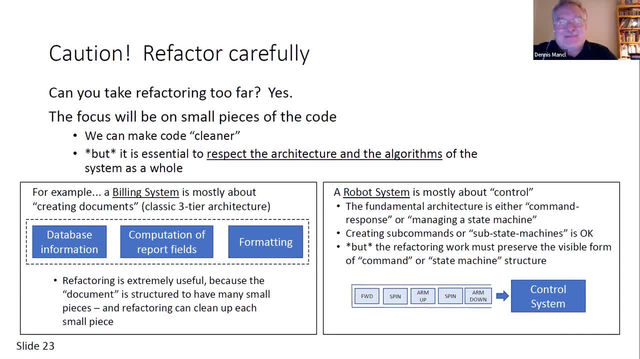 going to apply to my robots project, And I'm saying they always give the students the tough stuff right Because doing robot control is trickier. The fundamental architecture in robot control is usually either command response or it's some kind of state machine structure. 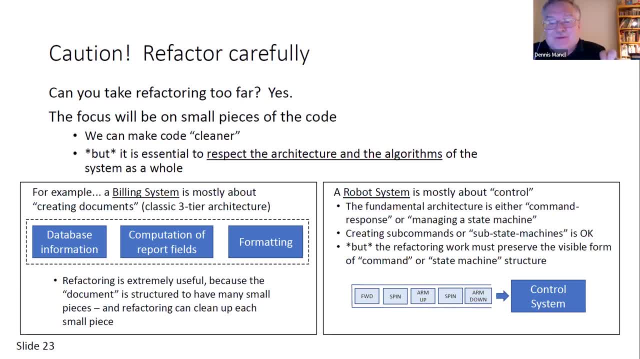 If it doesn't make sense to you, hey, don't worry. Certain kinds of refactoring Changes will be relatively safe, Things like creating some commands. Oh, I'm taking it, I'm decomposing this particular command into two or three smaller commands. 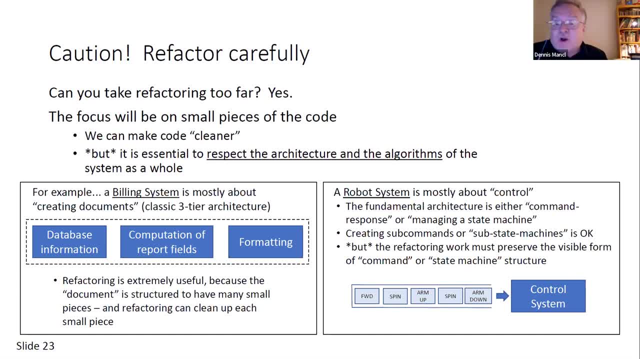 Yeah, Making sub-state machines is usually OK, But on occasion you may be trying to rewrite something that actually winds up hiding the main commands of the system. But don't fret: right When this happens, you will find that problem right away. 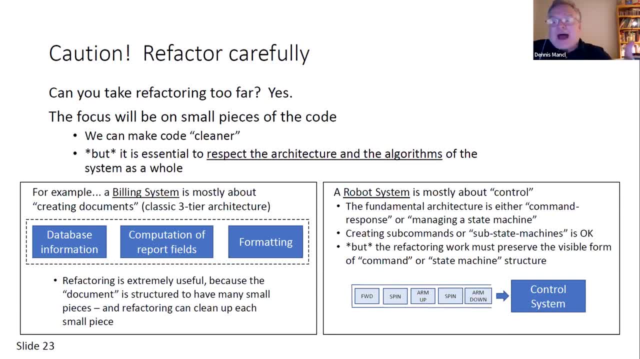 I assure you. And when that happens, you just back up to the previous version of the code before you made one of your refactorings and then try something else. Now backing up is OK. It's not a sign of failure, It's a sign of learning. 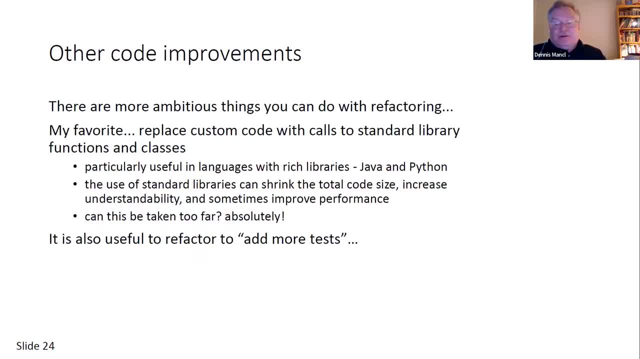 Cool, All right. There are other kinds of code improvements that you might consider. One of my favorites is increasing the use of standard libraries when you're working in Java or Python. Here you've got languages that have wonderfully rich libraries and well-tested, good and efficient code. 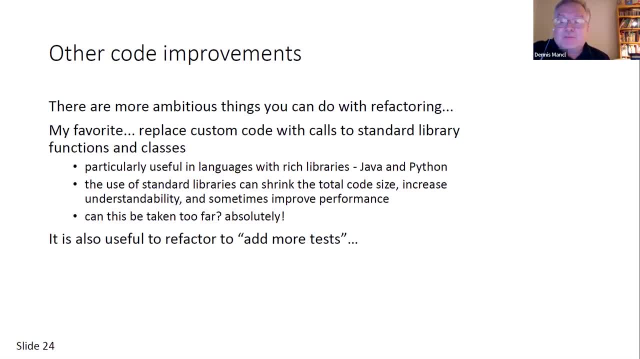 And for some reason, you didn't use it right. Agile developers sometimes forget to do things the easy way, And their friends should help them right. They should refactor to simplify where they can. Of course, don't go overboard. 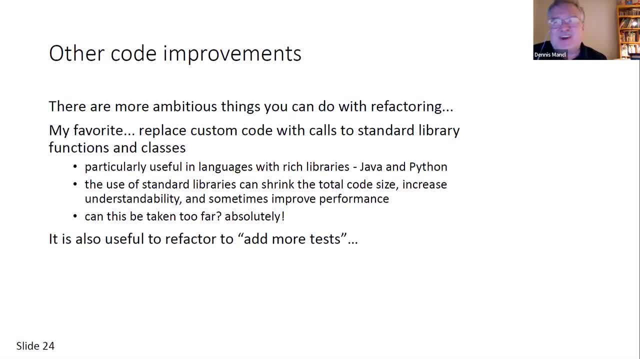 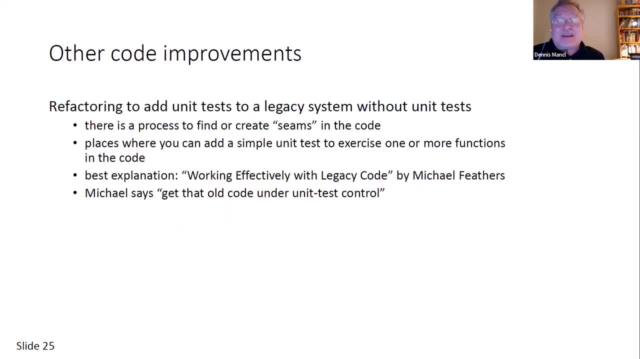 Can you say, oh, I'm training everything with the library functions. No, no, Use your JavaScript, right? It's also useful. another code improvement is to add more tests: Refactoring, to add unit tests to a legacy system that. 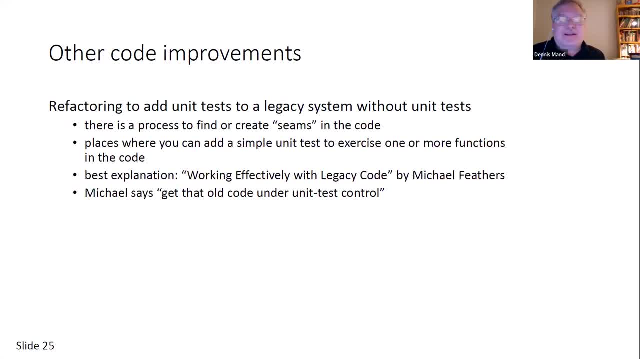 doesn't have any unit tests is a blessing, right? Oh, and it's a hard job, And I always point people to my favorite book on this topic, which is called Working Effectively with Legacy Code, by Michael Feathers, And he goes through lots of examples in here, in C++ and Java. 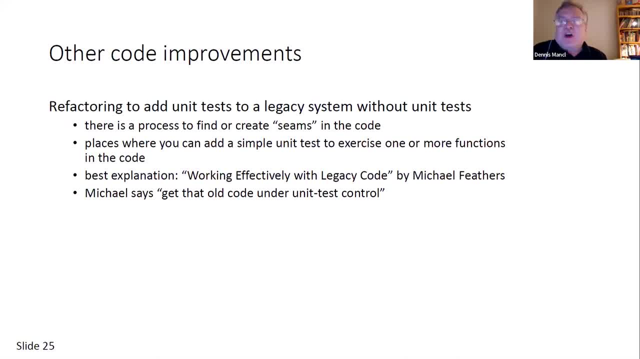 and shows various places. Well, one of the problems is you want to be able to drive a function in isolation from some of the things that are around it in order to have an effective and efficient unit test. And he shows you how you basically find the seams in the code and you basically 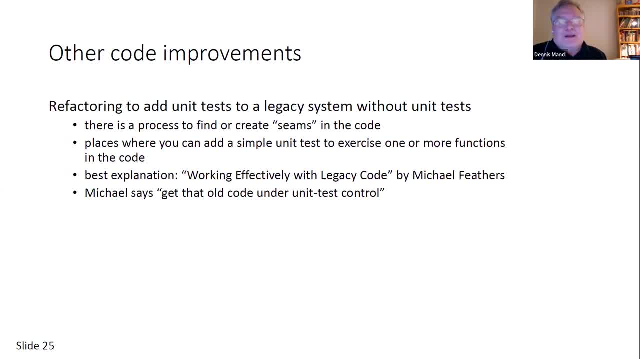 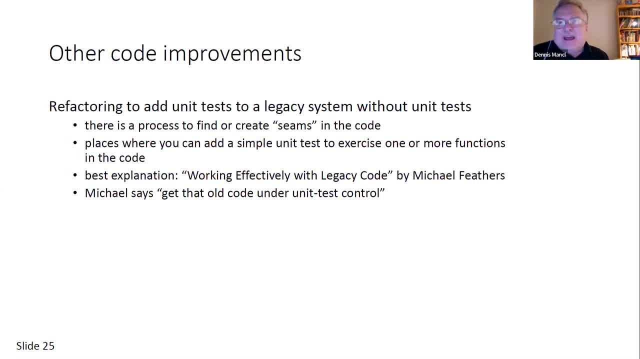 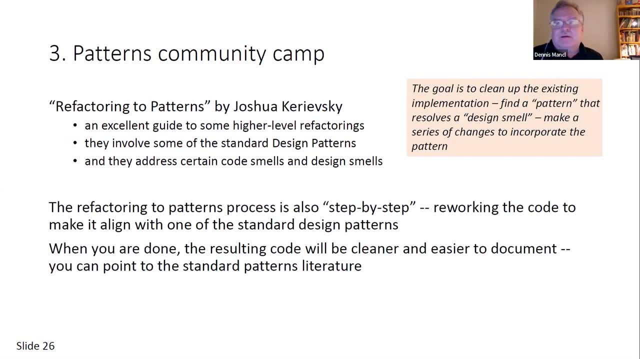 Get that old code under unit test control right? Spend a day every once in a while saying, let's improve our set of unit tests? All right. so now we're getting close to the end. here We're around to the patterns community camp. 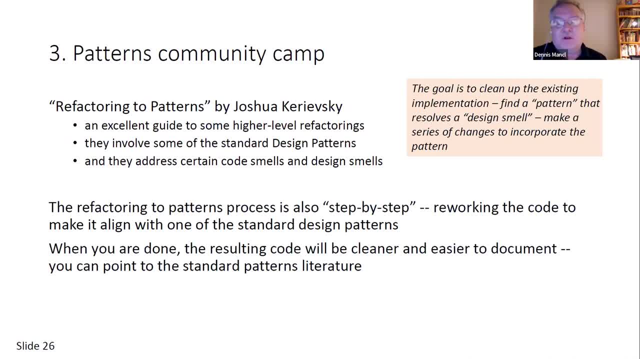 Camp 3 has a very different goal. Camp 1, remember- wants to make fixes and new code additions simpler, right? Yeah, we know we have bugs to fix. as maintenance programmers, We know that we're being asked to add new features. 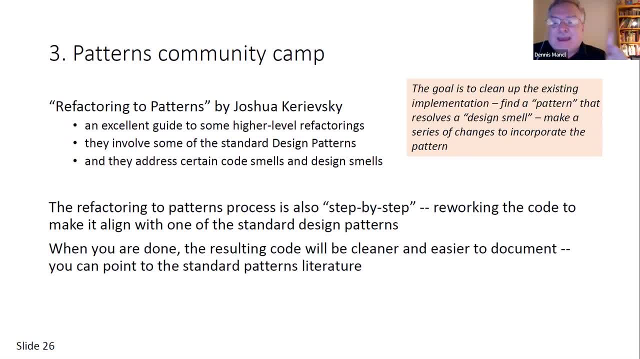 And we want to do some refactoring to help pave the way for that to happen. Camp 2 wants to support agile and iterative development, So they're doing a little bit of refactoring in every iteration. Camp 3 is about actually improving the design. 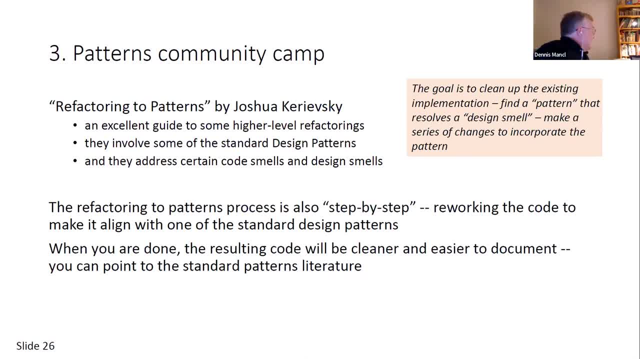 and, in particular, using some of the standard design patterns, And the book for that one is called Refactoring to Patterns by Joshua Kurevsky. OK, and in this design level refactoring camp, basically you have a different set of design, smells, things. 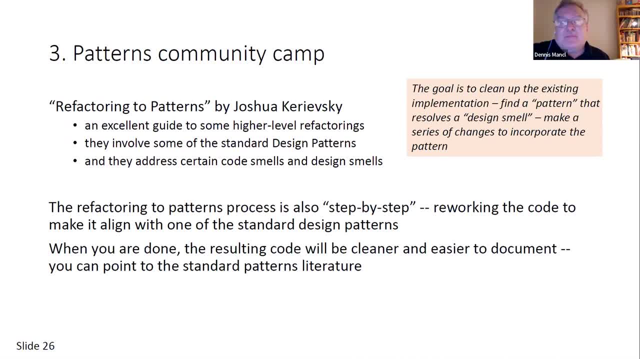 that you say, oh, I wish I could have done this differently, because I keep running into this problem when I want to extend this or want to debug that or want to test this other thing. So you find some patterns and you say what I'm really. 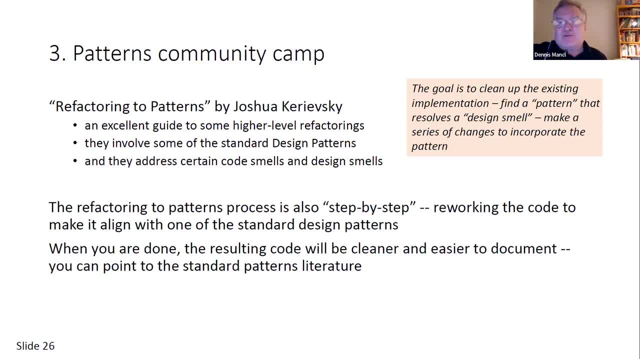 going to do is align my code so that it actually aligns to the patterns, And in some cases your code may actually be close. It may already be set up to use patterns like strategy or adapter or template method or factory method or command. 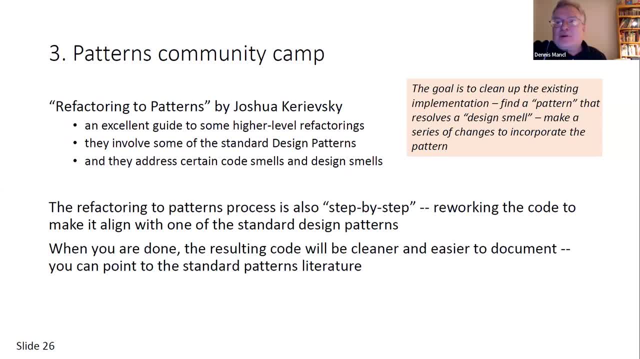 But if you make it clearer and you make it simpler and you make it very apparent that this is what's going on, there's going to be some positive benefits for the long-term life of your application. You need to identify the pattern and make it clear in the documentation of your code. 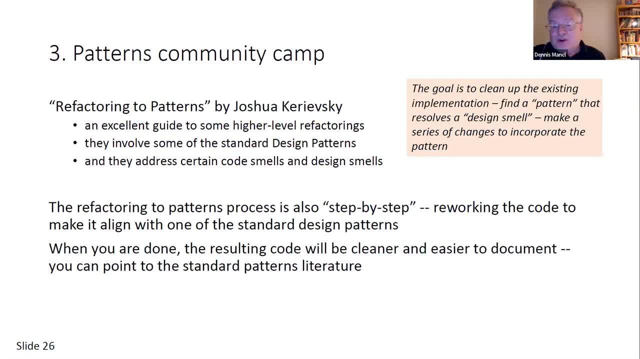 hey, I'm using command here or I'm using template method here, And then, once you get it documented, it's going to be more likely that the next set of developers that come along and are going to try adjusting your code they're going to look at this and they 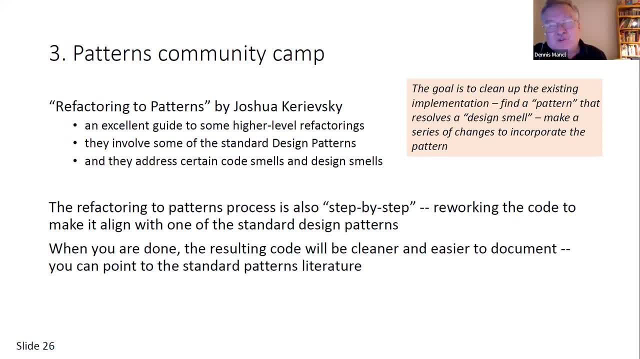 say: hey, this is actually a cool design. We're going to preserve that And we may actually be able to extend off of that. So it's a way to make the, The, The design, stronger and live more flexibly. So I got to show you an example in order. 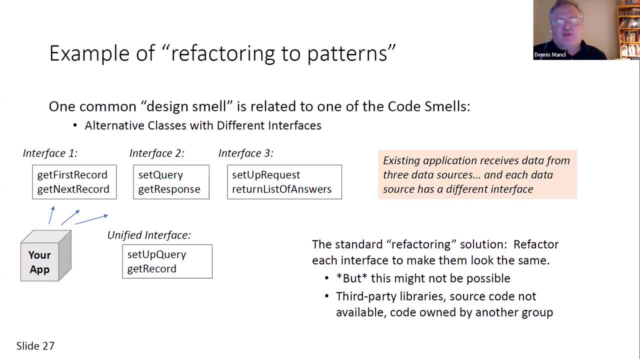 to make sure that you actually get this All right. So here's one common design smell that's related to a code smell. The code smell is alternative classes with different interface. Here we have different parts of this design were developed by By separate teams. 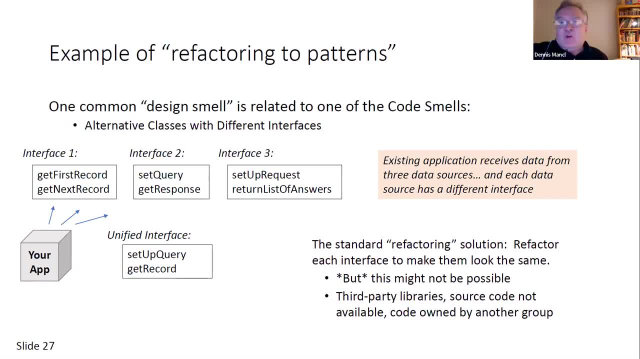 They often use different interface mechanisms in order to grab information from a particular data source. let's say, OK, they may be using an external library, so they're kind of forced into a particular style of interface. OK, so if you were doing ordinary refactoring, 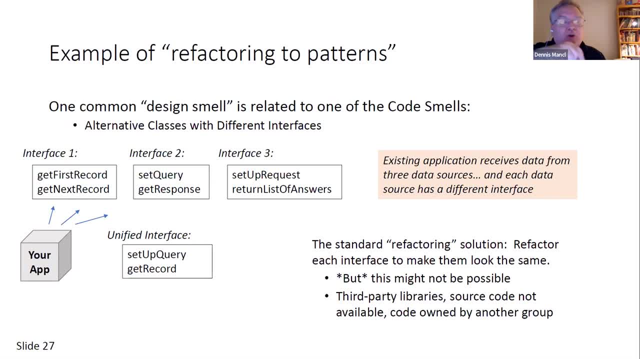 you're back in camp one, camp two, what would you do? You would say: hmm, I am going to take interface one, interface interface two, interface three. I'm going to slowly refactor each one of these three interfaces. I'm going to extract new functions, change the names. 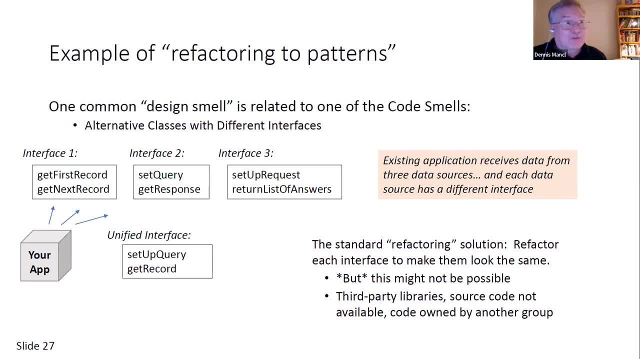 and eventually every interface would look extremely similar. They'd look like this unified interface down here. But maybe we can't do this, Maybe we don't have the source code so we can't change it, Or maybe another group, They own the code. 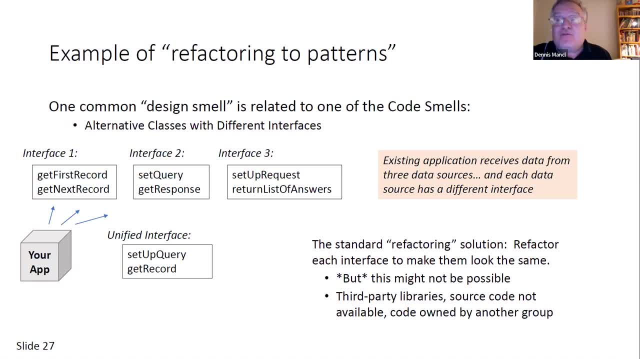 Maybe requesting code changes from them would start a big fight with another department. Oh so we may actually be in a situation where we're stuck with interface one, interface two, interface three. So what do we do? Well, maybe we use a pattern. 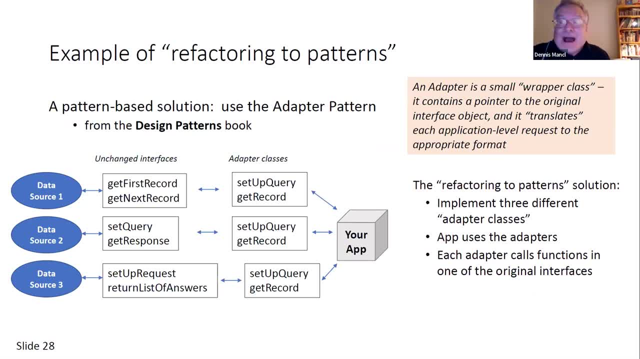 OK, well, it turns out. yeah, adapter pattern is made for this problem. Keep the three interfaces right. They're going to be the ones that are you're talking to and extracting information from the data source, But what you're going to do is set up three adapter classes. 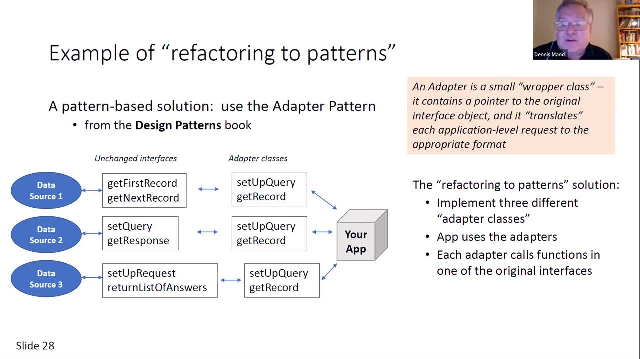 to communicate to those interfaces. right, And guess what? They're going to look kind of like this unified interface, And they're going to translate the setup query into whatever needs to be done in order to do the stuff in this interface one or interface two. 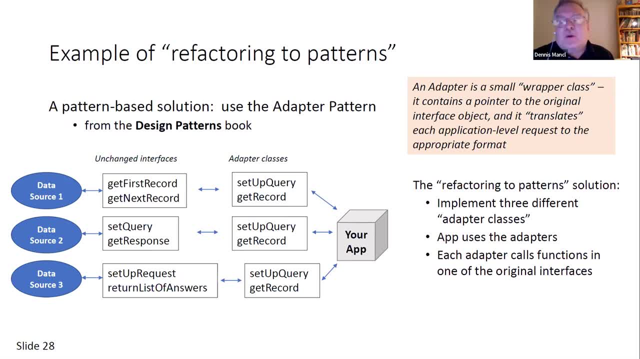 OK, so these are small helper classes that are built into your application, And it makes Things easier for your application because you can then slowly go through and unify all of the interfaces within your applications code, And the solution is not hard right. 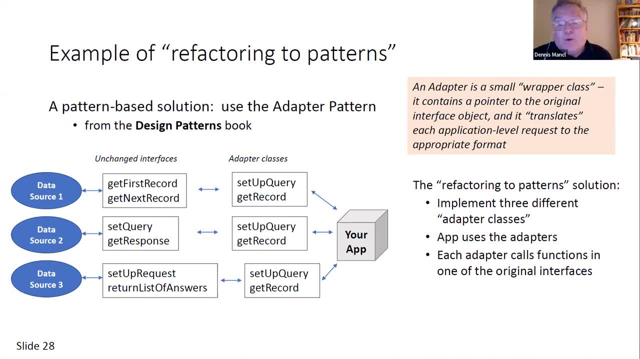 Adapters are easy to write. They're easier to change. We can work one interface at a time, go through and say we just need to explain what we're doing And when a new interface comes along in a new data source, we know what to do. 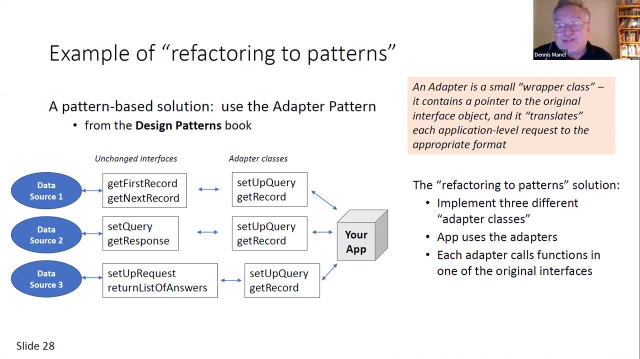 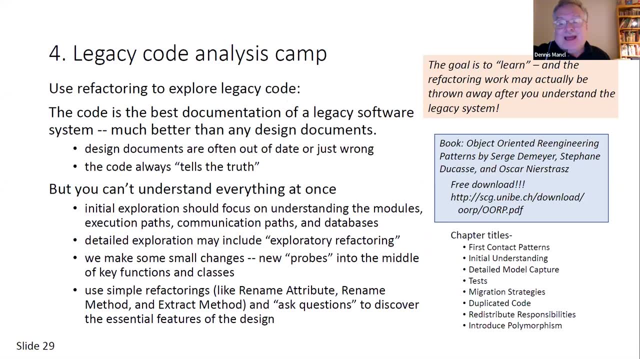 We say, oh, we're going to write another adapter, right, And it'll look the same, All right. camp four is legacy code analysis. And yeah, this legacy code analysis is a very different way of working with code. These people use refactoring in an interesting way. 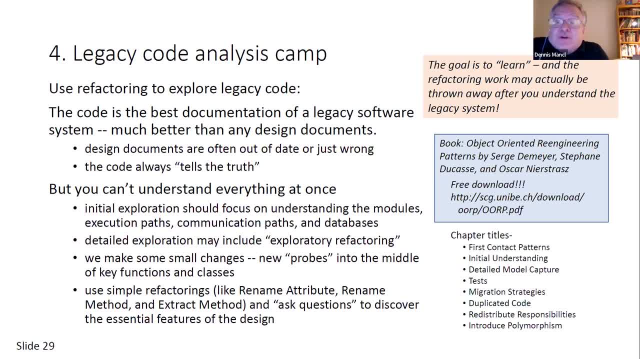 Their purpose. their idea is to use refactoring to learn. In fact, they might not actually make permanent changes to the code base. What they're doing, is they're going to do, is they're trying things out and asking questions. right, You're working with a code base that somebody else has written. 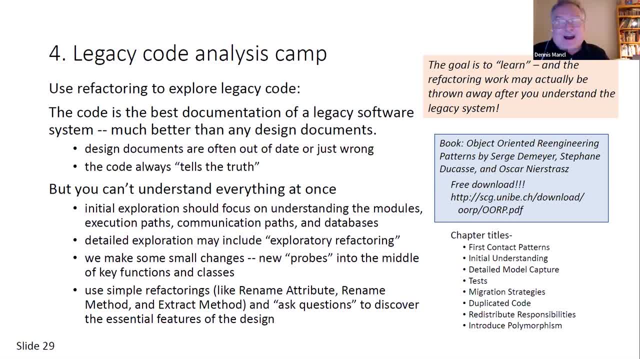 Maybe they're in another country, right? And you're trying to psych it out, And you're trying to say, well, how can I use this, How can I extend this, Where am I going to strip away? And you say I'm going to make hypothesis. 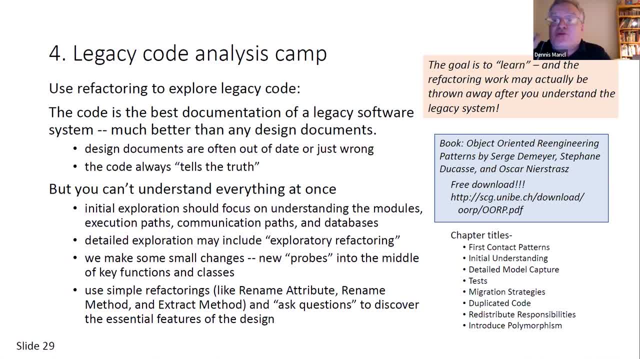 guess as to how the current code works, and then restructure the code to verify the guess, And then I'll put it back right And we do this. Why do we do this? Well, you say, well, we could read the design documentation. 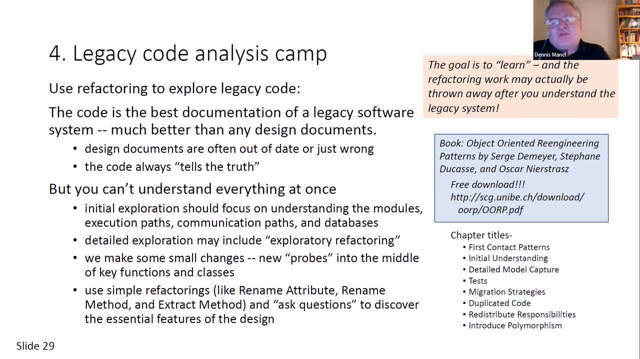 or we could read the code comments. But documentation and comments are not very good. Most design documentation for a legacy system is hopelessly old, out of date, wrong. The code is actually the best documentation. So to learn how to do this, I'm going to point you to. 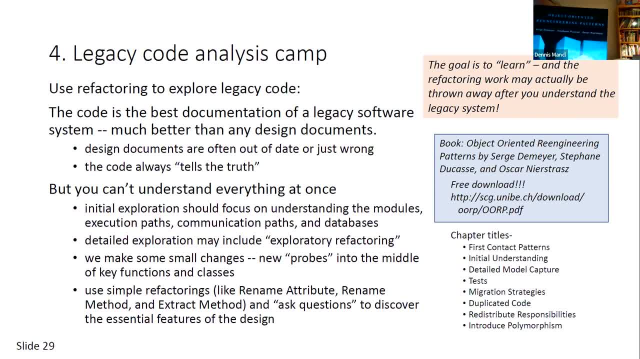 Yet another excellent book. This is called Object-Oriented Re-Engineering Patterns And it's written by these three Swiss guys, And I have the paper version of the book. But they said we like this book so much we're going to make it an open source book. 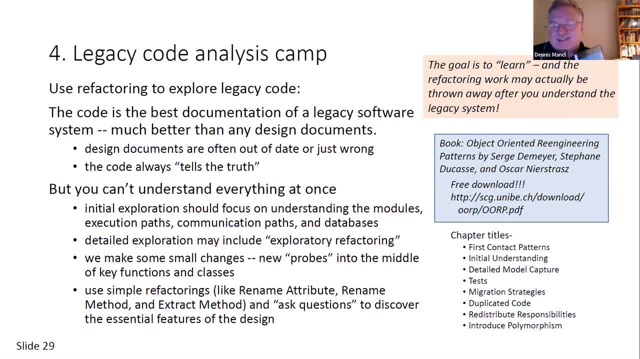 And they basically put the PDF file up on a web server someplace And they said, no, it's free now, You don't have to buy it, just download it Right, And it's an amazing set of tools And you'll learn a lot. 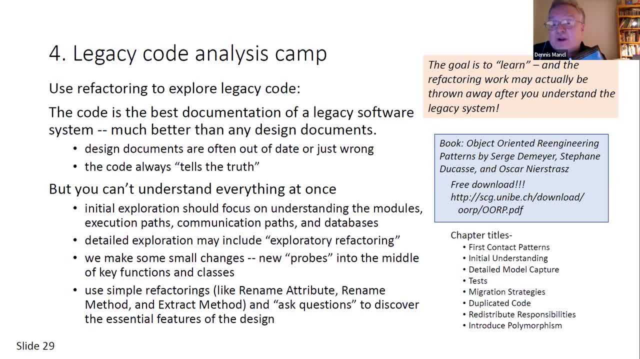 I'm including here on the slide the table of contents, the kinds of re-engineering patterns they have, And a lot of this is exploratory refactoring. You're putting new probes into the middle of key functions and classes, And they're all simple. 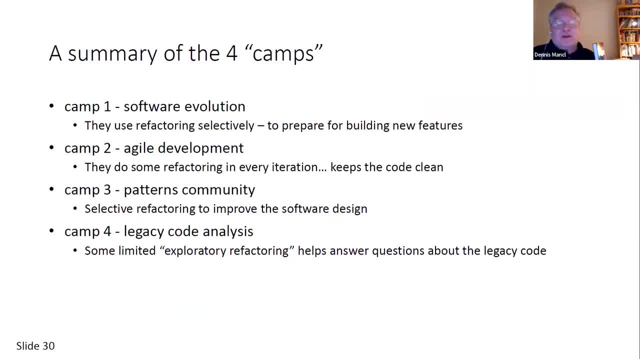 But they really help you understand your code better. So summary of the four camps: Right, We have Software evolution, Refactoring selectively. We have agile development, A little refactoring in each iteration. Patterns community: you're trying to restructure the design. 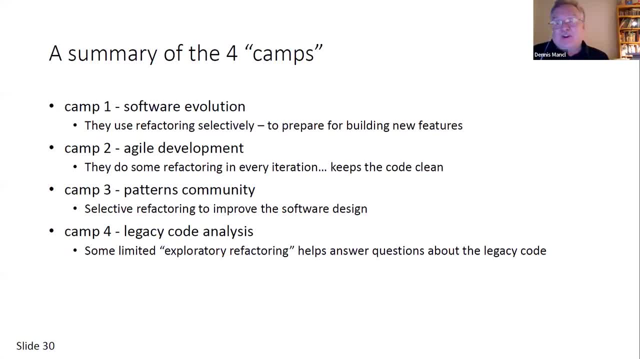 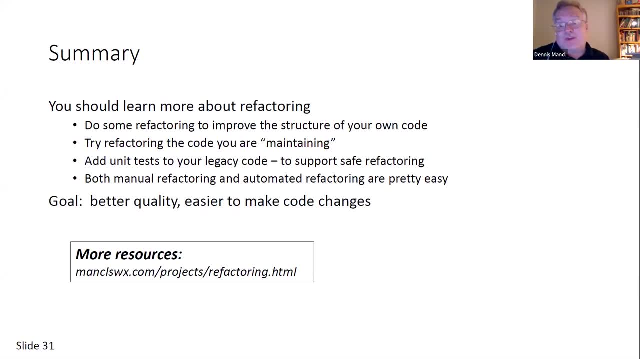 So it's directed. refactoring Legacy code analysis is exploratory refactoring. All right, Just about at the end Summary. You should learn more about refactoring, Right. Why should you refactor? Because you can improve your own code. You can make the code that you're maintaining better. 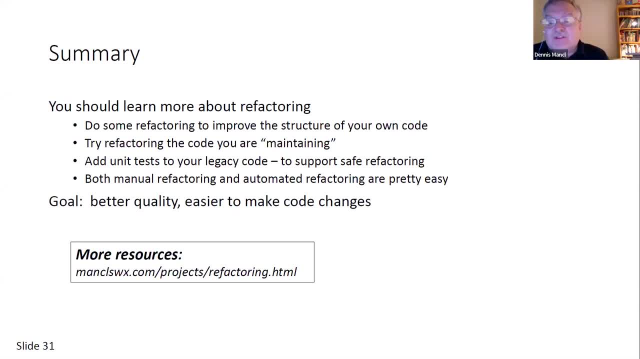 You can be more agile by including more unit tests, And this is not difficult, Right? Both manual and automated refactoring are easy. You'll get better quality, You'll get easier changes, And I've actually got a link here to some more resources. 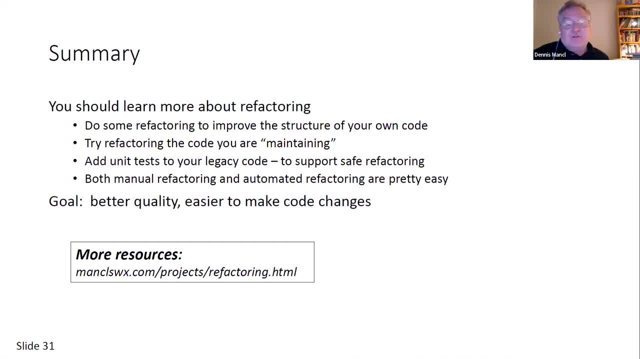 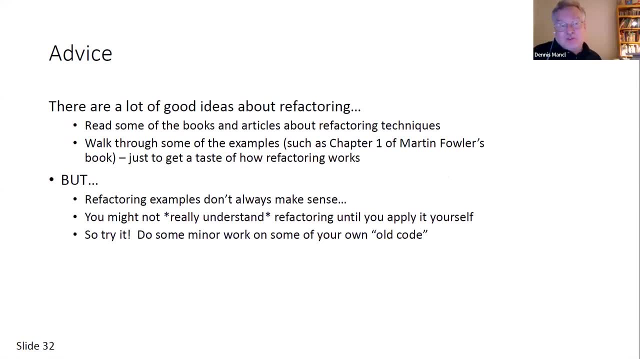 where you can learn basically how to get started on refactoring for yourself. One last parting bit of advice: You can learn a lot about refactoring from the books that I showed, from online articles, whatever, And it's good to look at some of the refactoring examples. 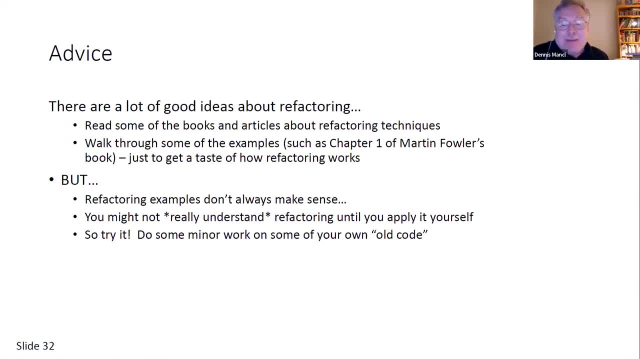 to get an idea how the process works, But many of us don't actually get it until we actually use the refactoring on code we really care about. So I suggest that you start with some old code that you have lying around. Anything older than three months is good. 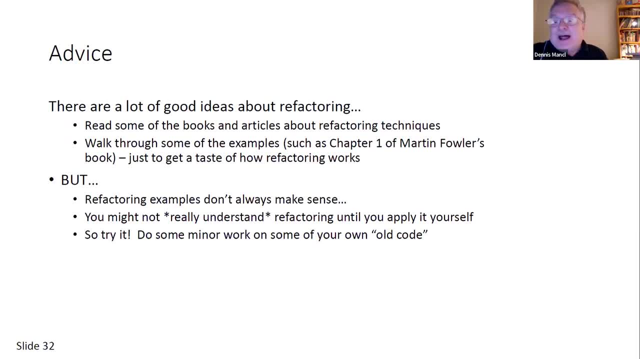 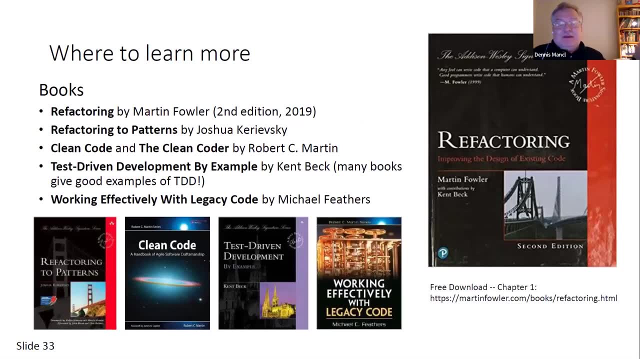 Right, You will learn something about refactoring and how to make the code clearer and more understandable. All right, And finally, here's some of the books that I referred to, And Martin Fowler's book is definitely a good catalog of refactoring ideas to try. 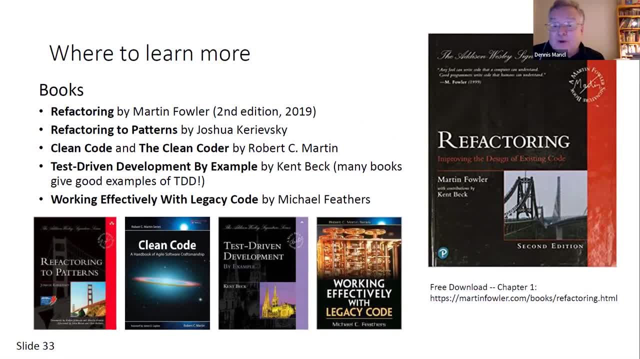 The Refactoring to Patterns book is more advanced, with some great ideas about design improvements. Note that a few of the books here don't even say refactoring And the title says refactoring. But they are right. Clean code is about making your coding style simpler.